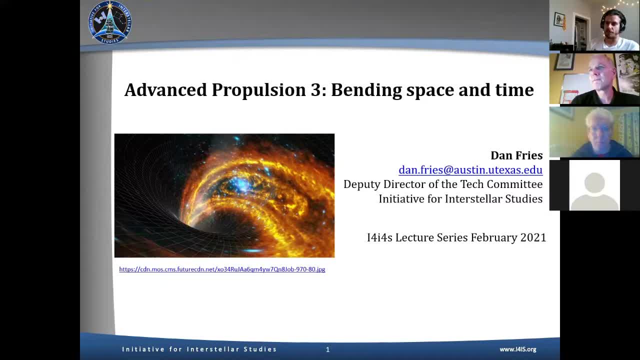 it's very fascinating, but you should take everything that's being told to you by me and also by other people when it comes to this kind of application, with a grain of salt, And we'll get into that, because this really gets to a point in our understanding of the natural. 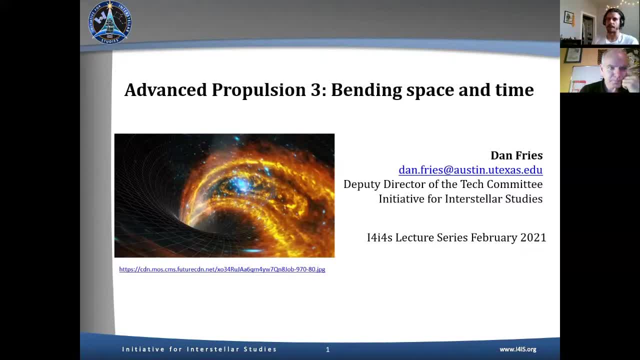 world where we are at the fringe of understanding and where the connection between relativity or the theory of space-time and the theory of quantum mechanics, the connection between them, becomes really important. And, as a lot of you probably know, this connection has not been made well, in some cases successfully, but in general, 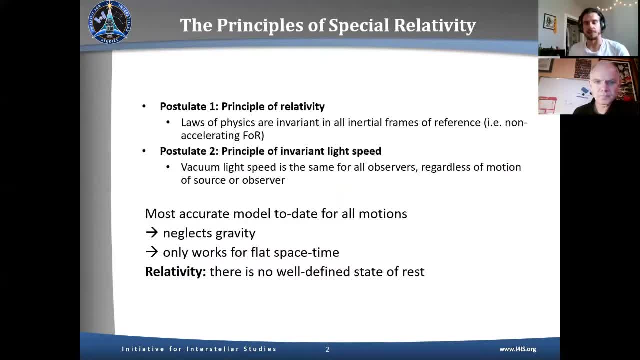 it has not been made successfully. So I'll just start with some overview of the principles of relativity. First with the special relativity, because that's the simpler case. And the two most important postulates of special relativity are that laws of physics are invariant in all inertial. 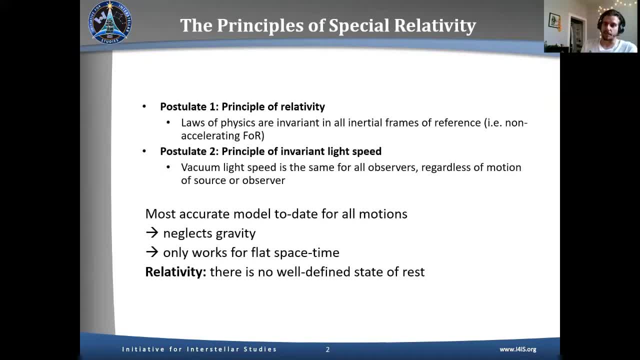 frames, and that light speed is invariant, meaning all observers, regardless how they move, they will always measure the same speed of light, And you probably heard this before, so you're familiar with these claims. What is important is that this approach 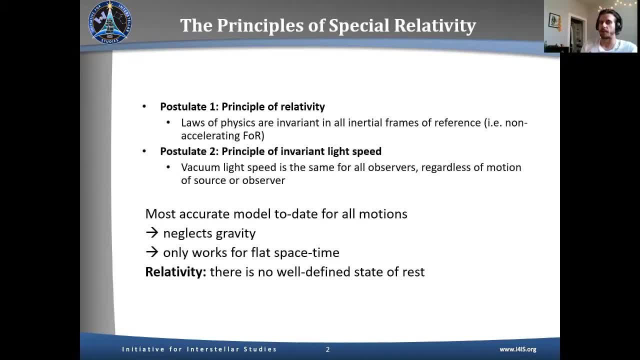 so far is the most accurate model for all motions that we've been observing. Special relativity neglects gravity and it only works for flat space-time and we'll get into that. And the name relativity comes from the fact that there's no well-defined 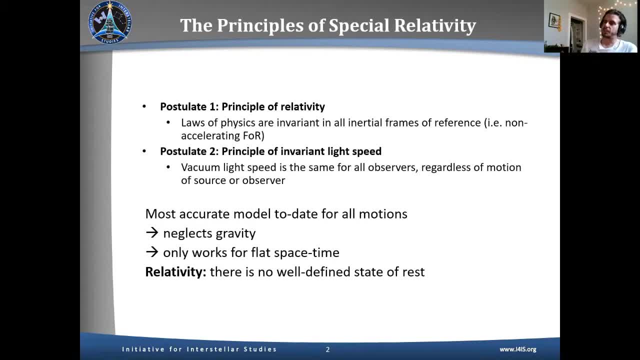 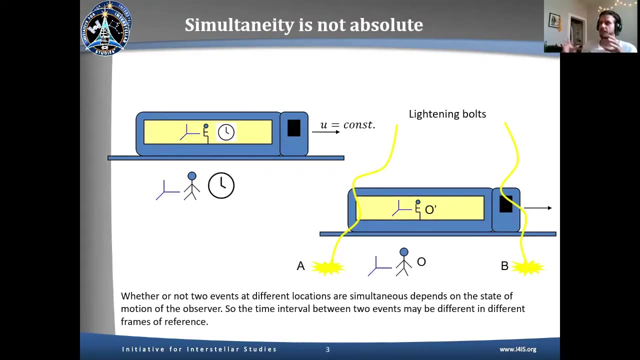 state of rest, meaning all the motion and observations are relative to the observer and how the observer moves in respect to other observers or other frames of reference. I'll give you an idea. So in special relativity, simultaneous events for one observer are not. 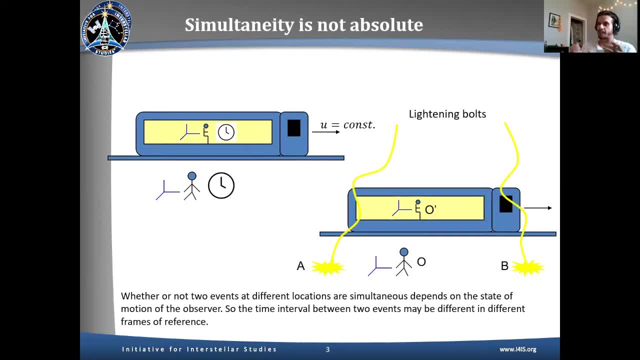 necessarily simultaneous for another, And that's like a classic example of what special relativity is. So if you look at these nice little trains, one person is standing here, the other person is in the train moving with a constant velocity. You have two lightning bolts hitting behind them and 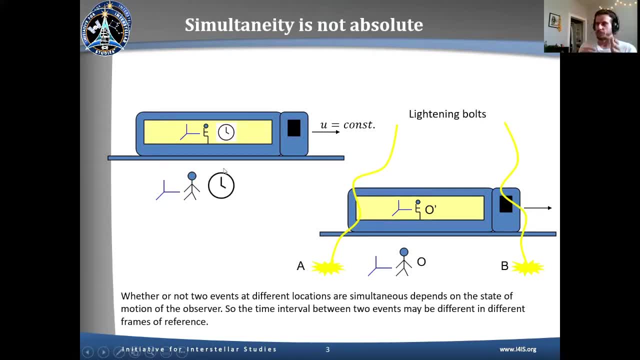 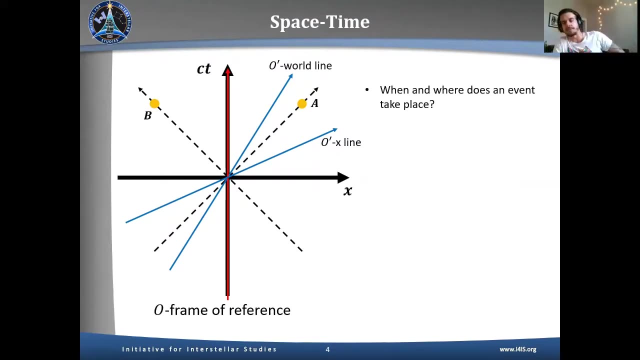 in front. The question is: will those two observers come to the same conclusion about where the lightning struck and at what time they struck? To answer that, if we have flat space-time, often we use something called the space-time diagram or Minkowski diagram, And I want to show you that because 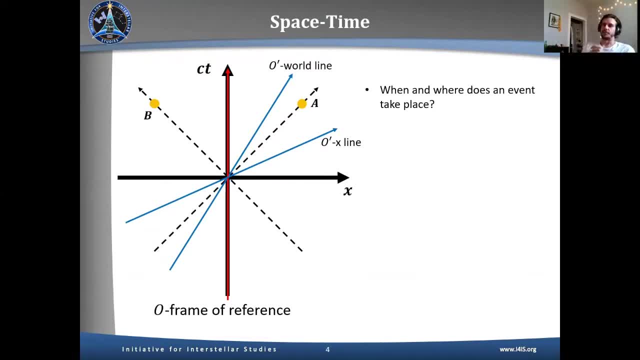 if you've never done this before, it's unlikely that you're going to get all of the implications right now. But I wanted to show you this if you want to do some more reading on your own, because it's a very powerful technique to understand the implications of special relativity. 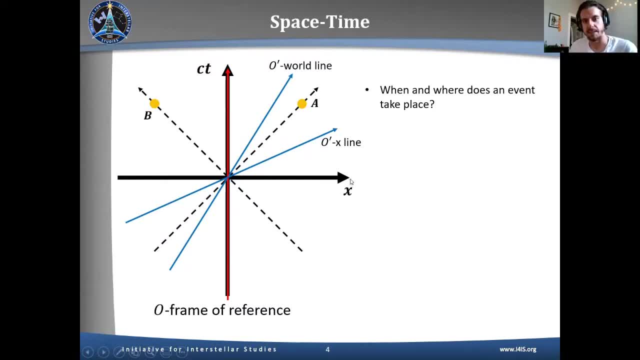 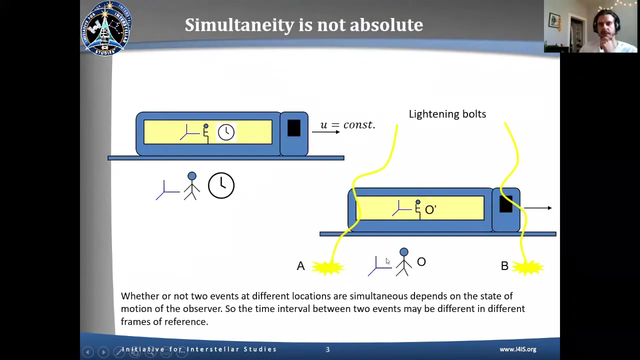 So you have here a spaceline- is x and you have a timeline- This is called the world line. often the speed of light times the time that is going by for the observer, And these diagonal dashed lines are the speed of light, And this black coordinate system would be our whole frame of reference. So if we go back, 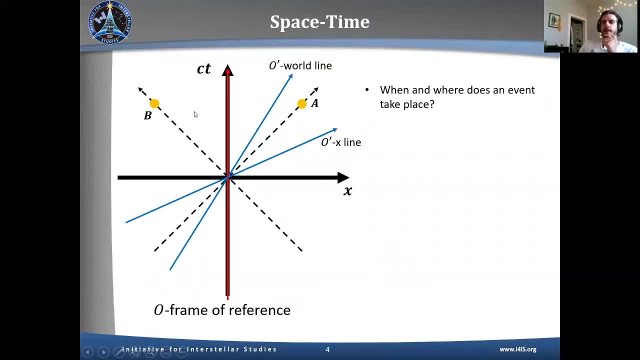 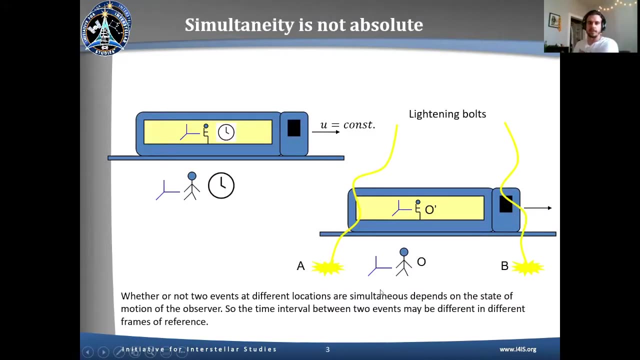 this is the unmoving character. And then we have a second frame of reference, which is O prime, which is this blue coordinate system, As you can see, for the observer in the O frame of reference, so the guy that's not moving. 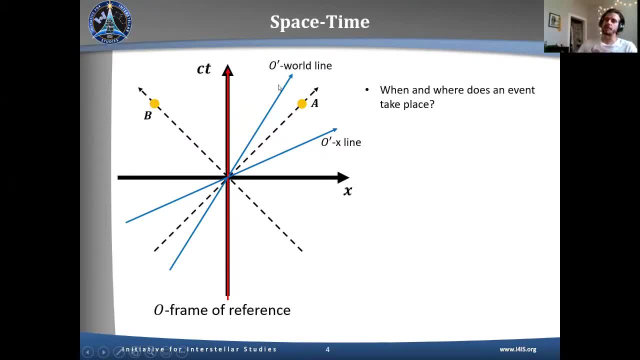 for him, the space and timeline of the moving observers look different from his own. That's because they're moving relative to each other. Now you have two events: the lightning strikes A and B, one in front, one behind- And the person, and they are on these dash diagonal lines. 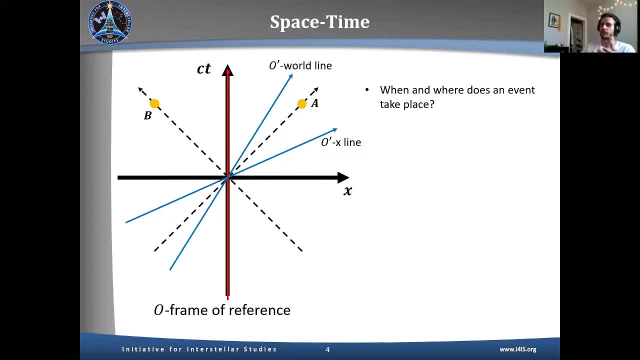 because the photons coming from these events are moving at the speed of light. And now the question is: how do these two observers perceive those two events happen? And what is important here is that Euclidean geometry does not give a consistent answer. In fact, we need the space-time interval. 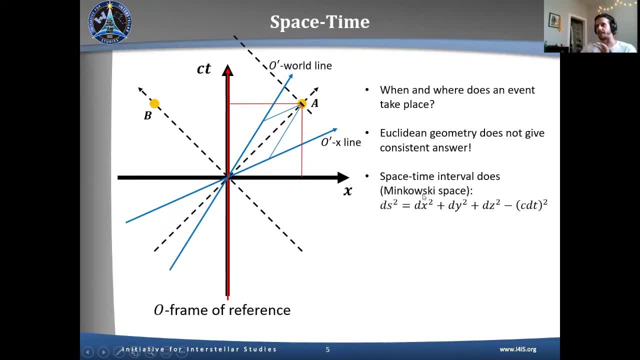 This is the Minkowski space, And that was the great insight that actually came after the first formulation Of special relativity: that space and time are not two separate things, but they're one and the same thing, And that's the insight that Newton missed. 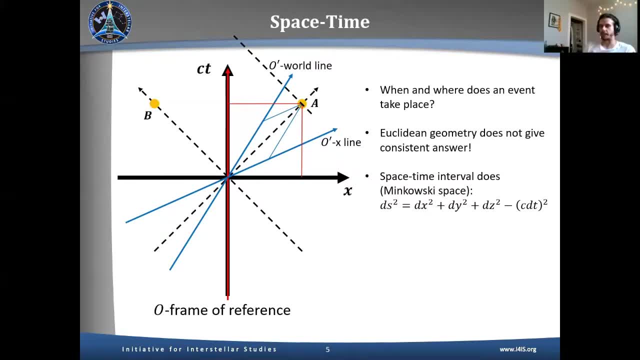 when he derived his laws of mechanics And that Einstein later had, that space and time are really one and the same thing. They are conserved, but individually they're different. And if we look closer at this event, the lightning strike A. 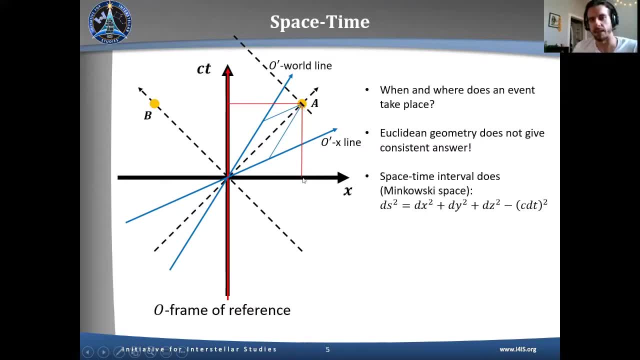 then observer O that's not moving would say: ah, the lightning strike happens here And I see it at this at this time. That's what he would predict. But for looking at the person that's moving he would say, well, 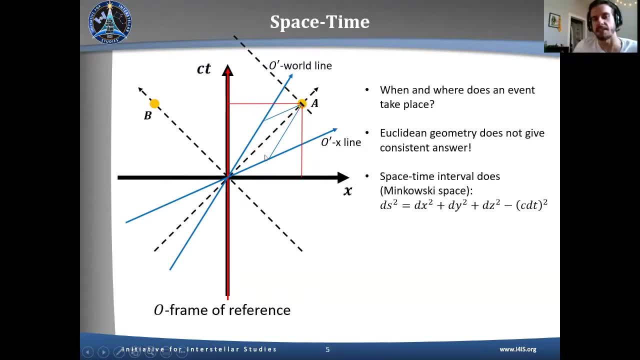 the moving person actually would see it at this time here at this place. And you can see that these distance and this distance, this, this or this time and this time, and this distance and this distance are not the same. So the two observers. 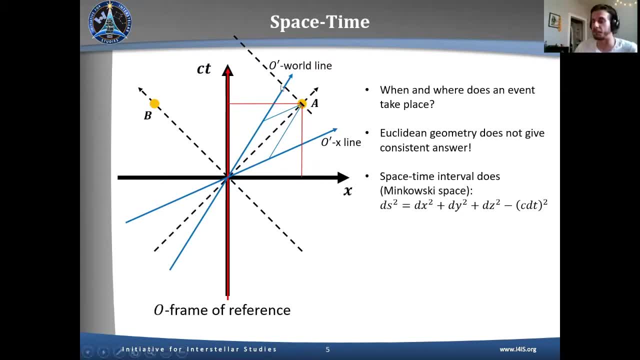 because they're moving relative to each other- would come to different conclusions. So we talked a little bit about this. Now, what happens- So maybe you've heard also what is inside of these diagonal lines here and below- is what we usually call the future and the past. 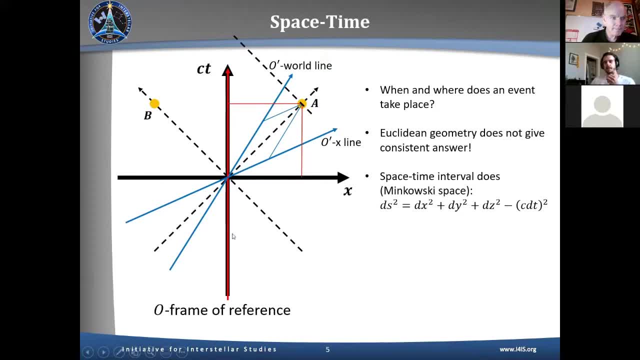 These are the light cones. So anything in here and down here can be, or has been, observed by our O frame of reference. Now what happens when we move outside of this cone? here We're below these diagonal lines, or above down here. Then we're in a range where something is moving faster than the speed of light. 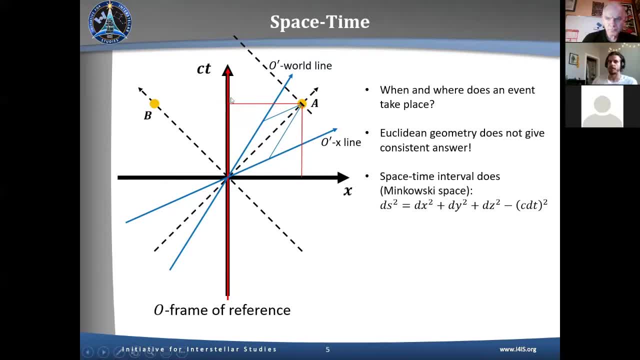 And it becomes causally disconnected from the rest of the things happening here And in fact it cannot influence and it cannot be observed by the person at the frame of reference from. from that notion You also can define an event horizon, anything that's in this area. 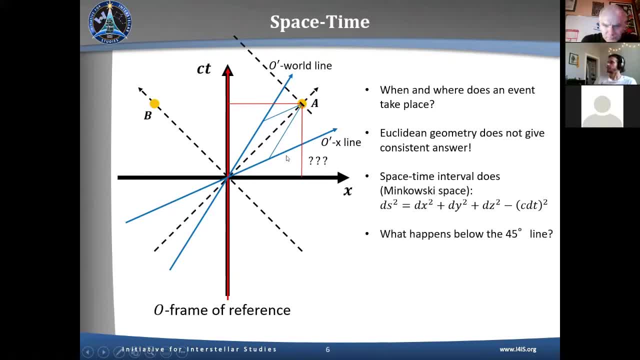 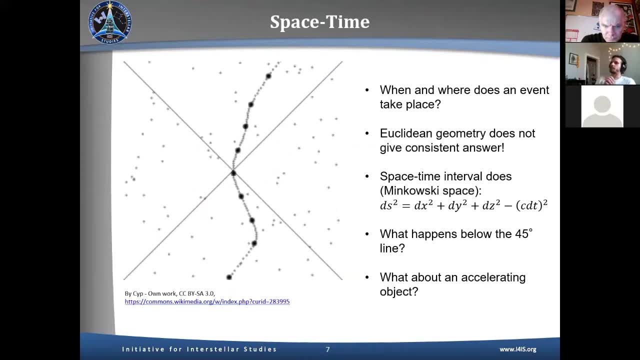 you would not be able to observe. So the next question is: what would happen if you are not moving with a constant speed, but you're actually an accelerating observer? Well, in that case, what you can observe and what can influence you is constantly changing. 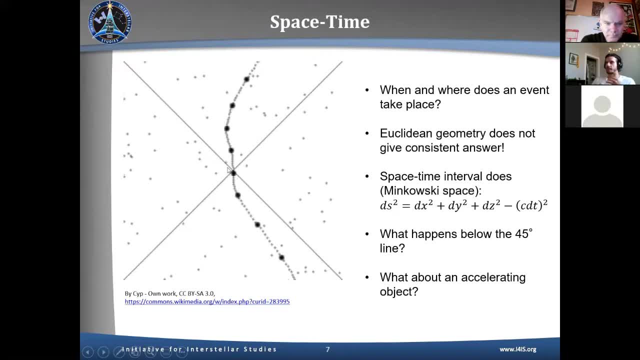 So here we are, in, accelerating, observer, So non-inertial. and these pluses and dots they are. well, the dots is our trajectory and the pluses are events happening somewhere in space and time around us. And if we're moving at a constant velocity here, 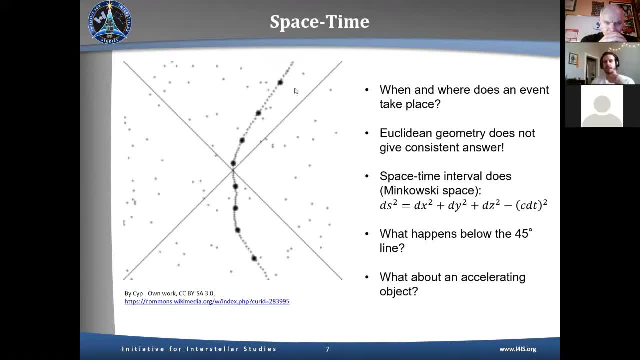 nothing shifts. it's just moving down as time goes by. But as we're accelerating, you can see that some of these events move below the diagonal lines here or they move from here above them, And that means that, as we're accelerating, the events that can influence us and 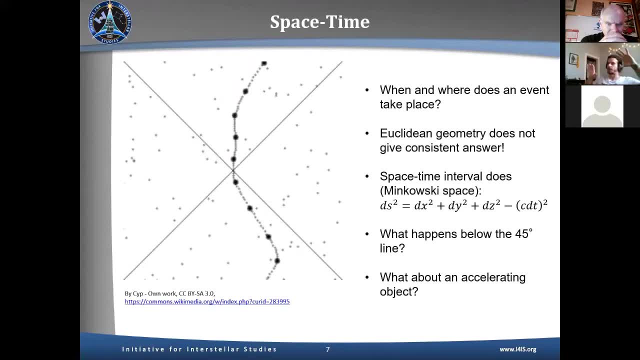 that we're observing actually shift in and out of our light cones And again this gives rise to the notion of an event horizon. But it's very interesting that, as an accelerating observer, there's basically as you change your state of motion relative to other things in the universe. 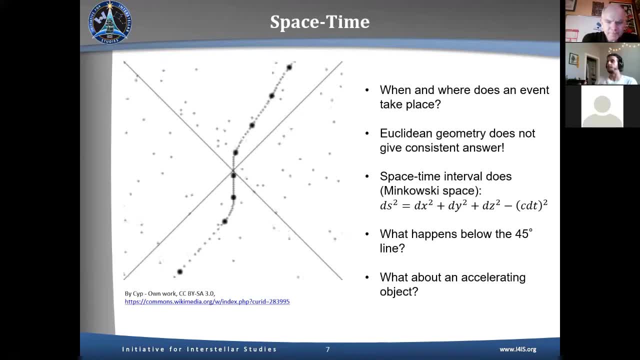 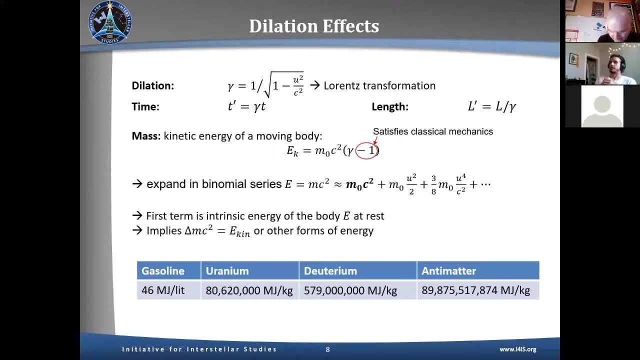 the things that can influence you also keep changing This. all of this, what we've talked about, the relativity of the location and the time interval between events- gives rise to the notion of the diagonal line, And this is the notion of the dilation effects. 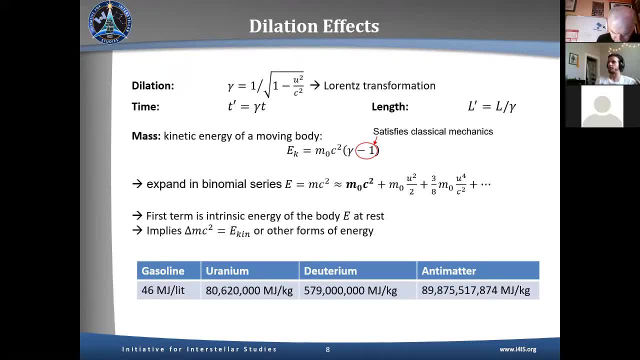 You probably have heard about that too, maybe through the twin paradox that if somebody is moving fast, that for them time is going slower than for the observer at rest. It's a little bit simplified, but let's leave it at that. This dilation can be quantified with the Lawrence transformation. 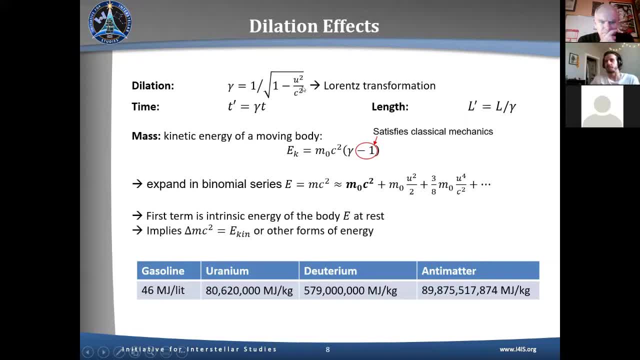 which is this factor here, And it's mostly just a function of the velocity at which one is moving, divided by the speed of sound squared, And time is dilated in this fashion. So if somebody is moving fast away from me, then for me. 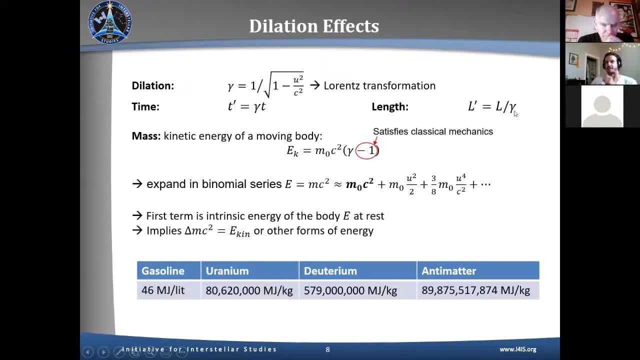 it looks like time for them is going slower. And at the same time, if somebody is moving away from me fast or even towards me very fast, then it looks to me like the physical dimensions of an object are contracted. And again, if we would do this in a space time interval, 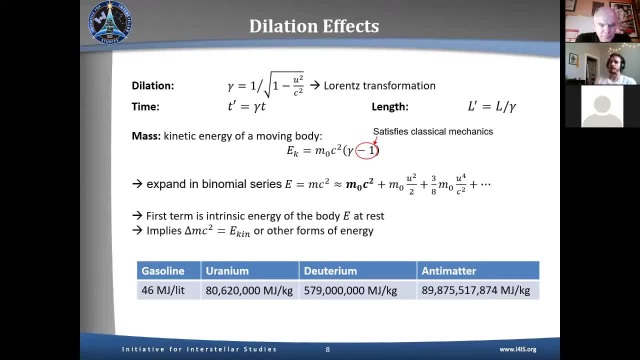 nothing would change, Then everything would stay constant. Um, but if we're looking at those two quantities separately, then they, they change, And this dilation effects then plays into the derivation of Einstein's most famous equation. I just wanted to show this. 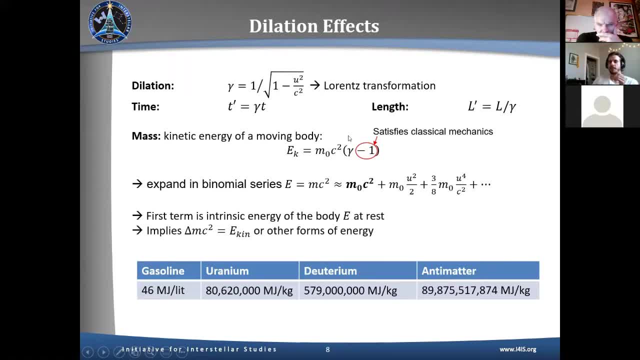 So he originally derived the kinetic energy of a moving body as this equation And this minus one factor satisfies classical mechanics in the limit of no motion And M zero is the mass of the body at rest. If you take this and you expand it in a binomial series, 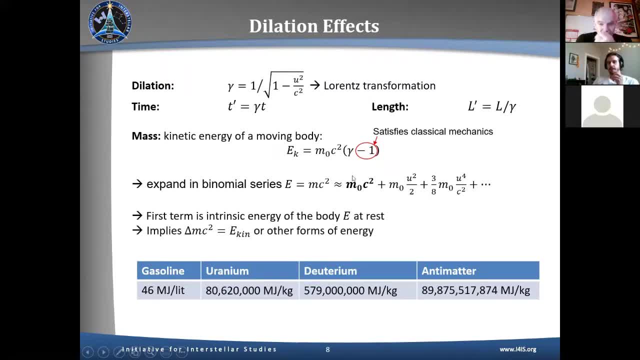 you get this year where this is the, the key result being that the that an object has an energy, even if it's in rest and intrinsic energy, in that this rest mass is equivalent to an energy of this body, And it also implies that every other type of energy that you add to the body is actually equivalent to maps. 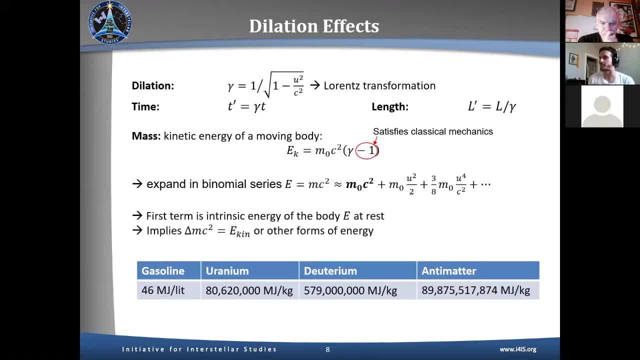 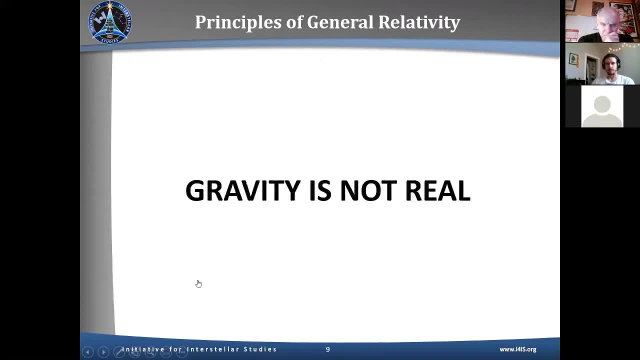 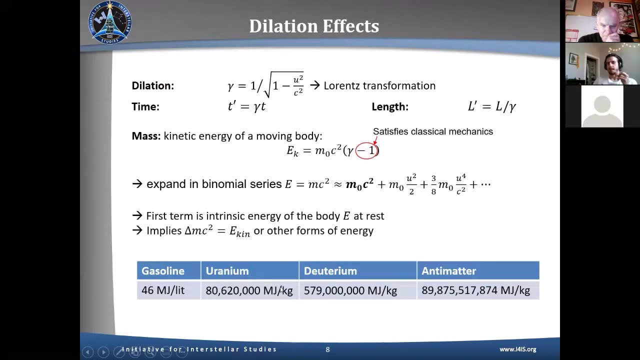 And so you get the notion of relativistic mass, where an object, if it's accelerating, it's mass starts increasing, And of course it also shouldn't click here- gives rise to the idea of the atomic bomb. If a per kilogram uranium 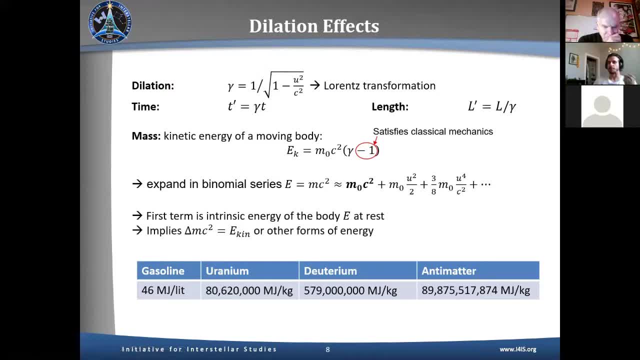 if you get a certain, if you extract some of the potential energy out of this you get, you can create a very destructive or very energetic device. Let's say, with the peaceful stuff you can build a very good power source And 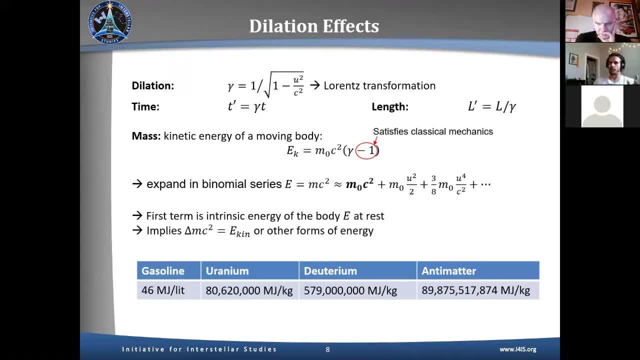 the more of this internal energy of a molecule you can convert, of course, the more energy you get out of it. Now, uranium, this would be just burning something, So you release some of the bond energy of the molecules, which also manifests itself as mass uranium. 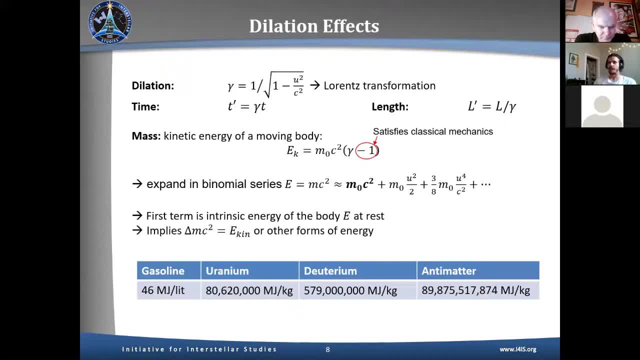 you have fission, So you get a bond energy between atoms. Deuterium, that would be for fusion. So again, that is a. that is a. you can only do that for specific atoms where the energy difference is such that you get some energy out of it after you fuse the atoms. and anti-meta, of course, would be the complete conversion of the rest mass itself into energy. 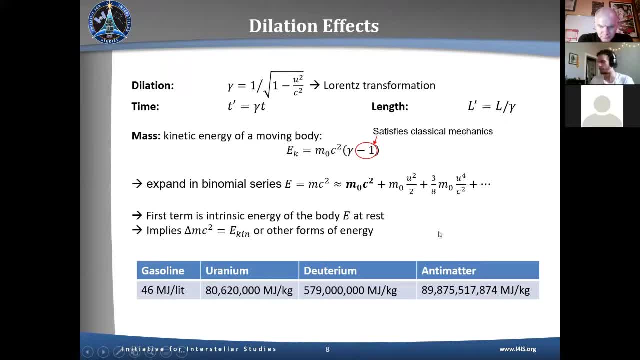 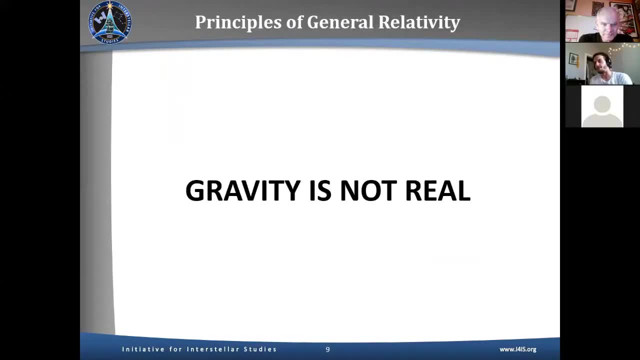 which is the one of the most efficient processes. very desirable, but haven't been able to do it yet. Now, when we move to general Reddit relativity, I like to start with this statement that gravity is not real, And the first time I heard about that. 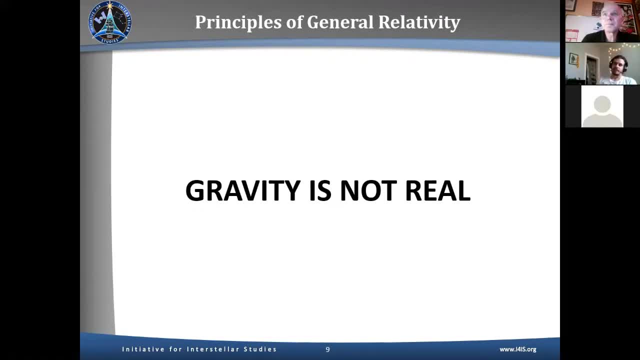 it took me some time to wrap my head around this- that in the context of general relativity, you can basically treat gravity- gravity as a fictitious force, the same way you would with the centripetal force or the Coriolis force. 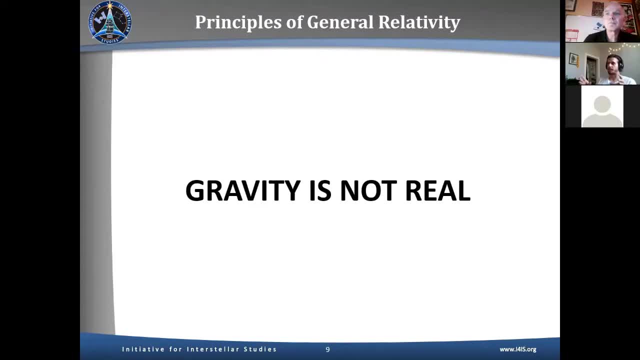 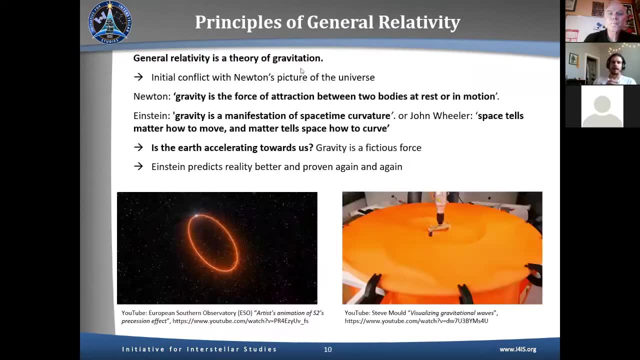 It only exists in a frame of reference that is subject to a space time distortion. If space time is flat, there would be no gravity. So this has been. this has been discussed at length because it was a huge conflict with Newton's picture of the universe. 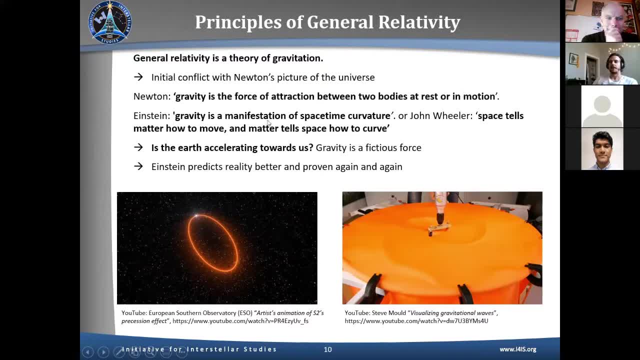 You would say gravity is the force of attraction between two bodies. And then when we get to general relativity, the idea is that gravity is just a manifestation of space time curvature. And then grab, we can say gravity is a fictitious force. 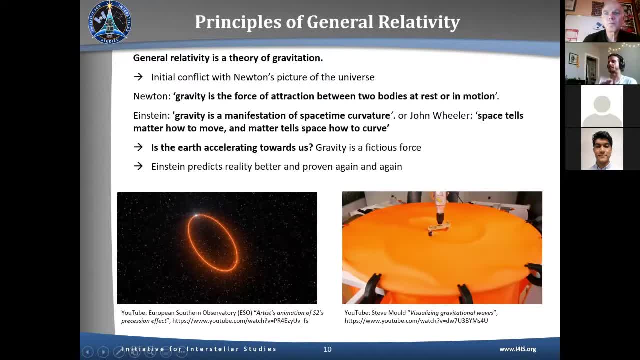 because in this context, you can look at us staying on the surface of the earth, not as a result of a force acting on us, but as the fact that the earth's surface is constantly accelerating towards us- which is when I've heard it for the first time- was pretty mind boggling. 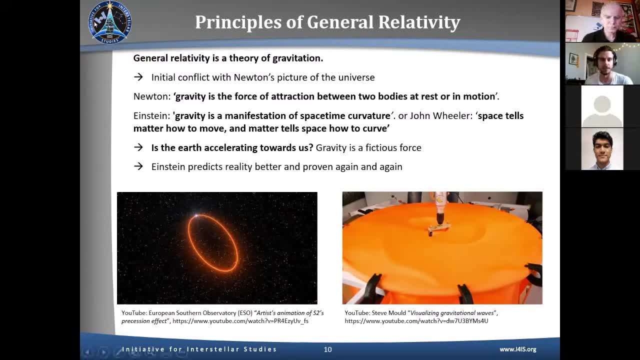 I think this is one of the most interesting outcomes of these theories. General relativity: Again, this has been one of the most it has been the most successful theory of you to explain the motion of, of a macroscopic objects in the universe. 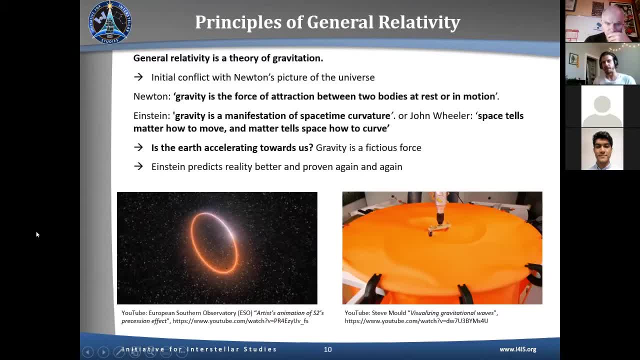 It predicted successfully the procession effect that we see in the stars moving around black holes, something that Newtonian mechanics is not able to predict, And you can see this here in a nice little simulation. And it also predicted gravitational waves, which only recently we started to observe and where the 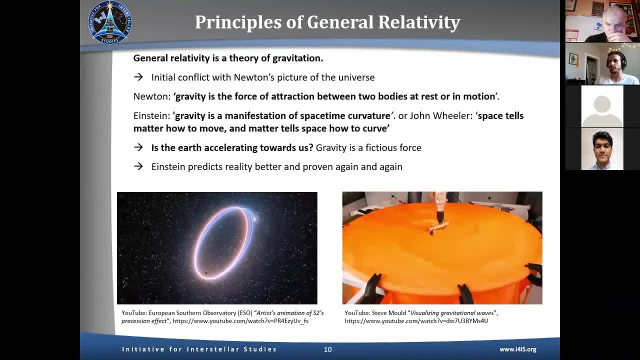 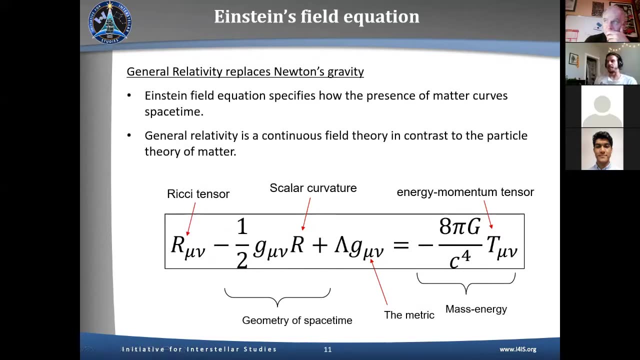 where the implications and potential for research is not, is not completed by any means. All right, So to give you an idea again, this is not necessary to talk about some of the propulsion concepts, but to give you an idea of the different concepts that go into general relativity. 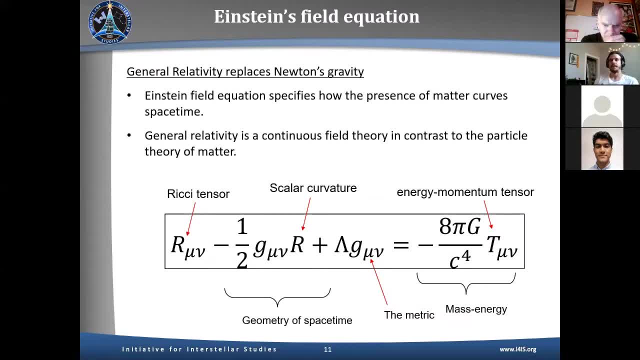 and maybe also so you can look at stuff that people present to you and you have a better understanding what they talk about. the general relativity: When we replace Newton's gravity or Newton's loss of motion, we need the Einstein field equation. 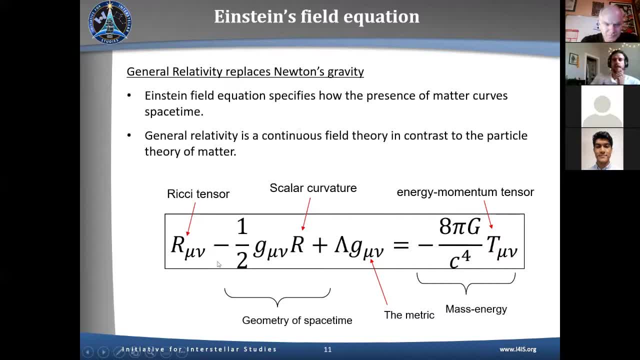 And this is a continuous field theory. What is important in this equation here is that you have a geometry of space time encoded in this term, You have a metric which describes how you would move along this space time And you have an energy momentum tensor. 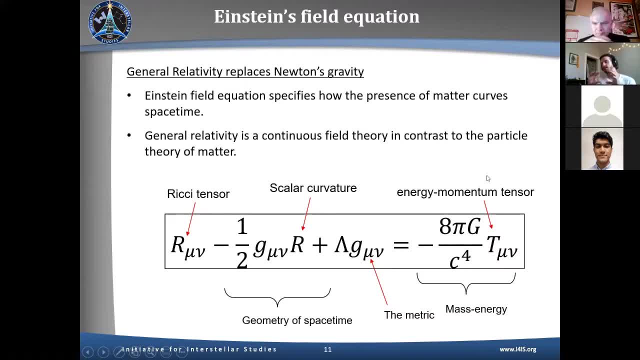 And this whole term on the right hand side here describes the massive energy distribution that gives rise to the geometry of space time and the way that you have, the way that the space time interval is curved on this space time. So this is where the equivalence between space time curvature and the distribution from energy and momentum comes from. 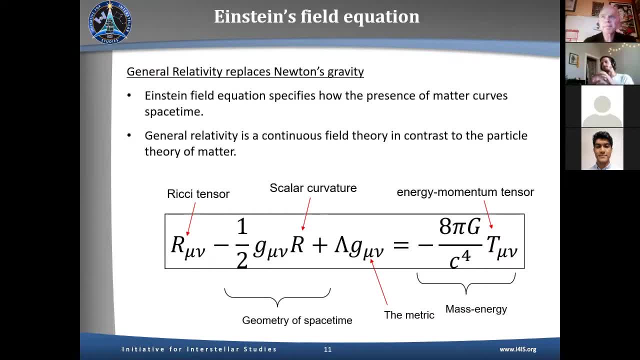 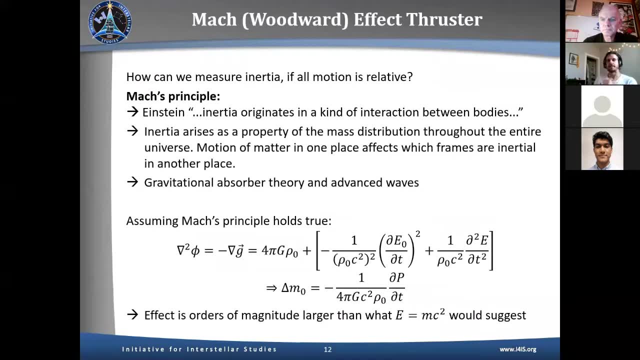 All right. So now we have some basics. I'm going to move into application to space Propulsion And I want to start with one that is actually being tested, and it's called the Mark effect thruster, Although now I think a lot of people would call the specific effect that is used to produce thrust. 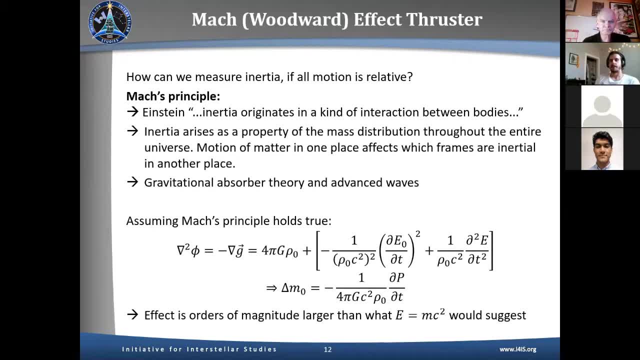 The Woodward effect, after the person who is currently performing most of the research on it, and the Mark effect is originally tied to a very particular function of the Mark effect, And so we have a very specific function of the Mark effect that is used to produce thrust. 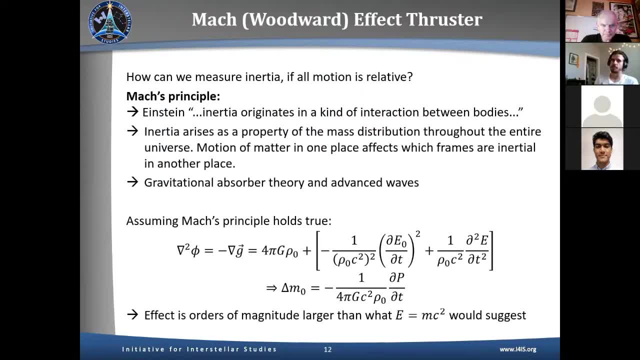 which is the Woodward effect, And I think that is called the Mark effect, And I think that is the Mark effect, a problem that still, that still has not been solved, and that is so we have a rest mass and we have inertia in the einstein field equations and they do stuff. we can describe what they do. 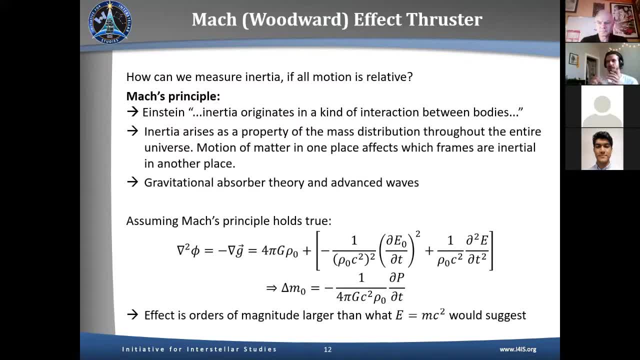 but the underlying question of how does the inertia actually arise is not solved. if all motion is relative, then how is it possible that we have any kind of absolute inertia? and so mark's principle basically says the inertia comes from the interaction of a body with the mass distribution of the entire rest of the universe. 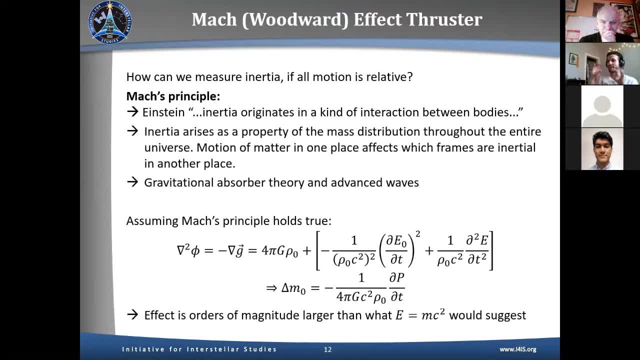 um, now this is. there's a lot to swallow and there's a lot of- uh, i would say- discussion still going on, because to make this work theoretically you have to rely on stuff like gravitational absorber theory and advanced waves, which is still active fields of research and where the 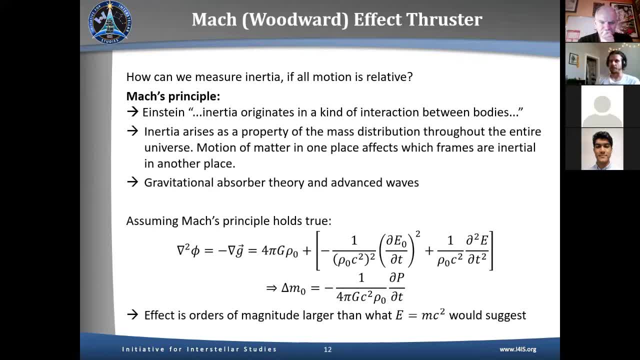 last words have not been spoken. so especially with advanced waves. uh, this is a topic of of discussion. uh, that's not settled. but if you accept that mark's principle is true, so that the inertia of one body arises due to its interaction with the mass in the rest of the 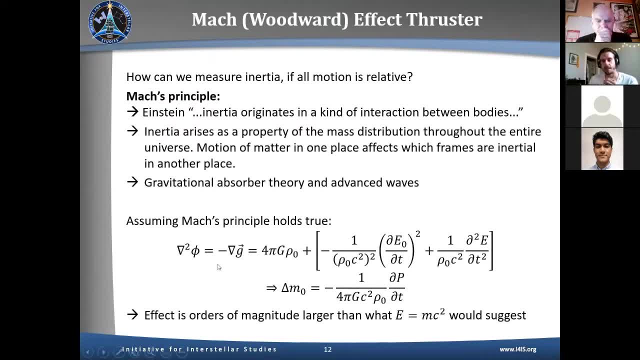 universe. um, you can, can write out a gravitational potential equation, which is here the first one in which you have higher order terms. so this first one here, this four pi g, rho zero, would be corresponding to your rest mass, uh, influencing the gravitational potential. and then, on the right hand side, you 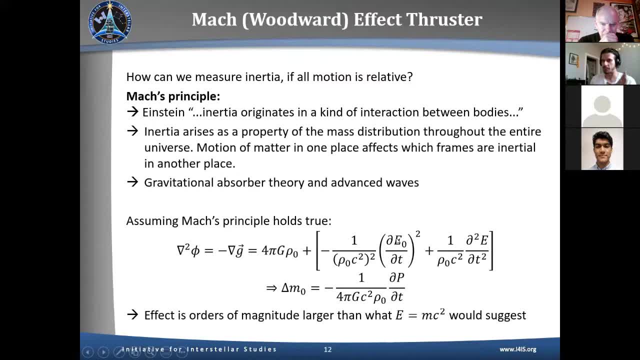 have higher order terms, where fluctuations in an object's energy can introduce fluctuations in the gravitational potential or, vice versa, fluctuations in the object's mass. and if we neglect this first term here because it's low order and usually very small and you integrate it over a power cycle of some device, you can. 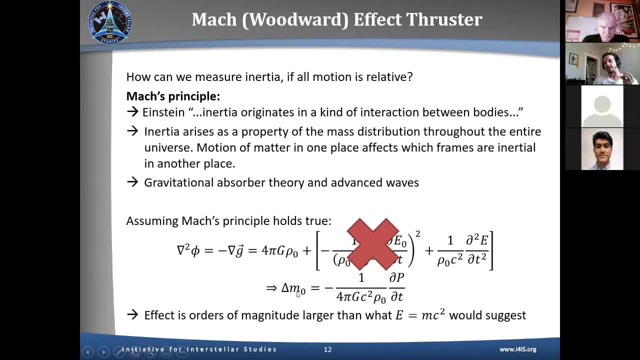 actually write an equation like this where you have a delta in rest mass um equal to negative, some constant times the time change in power. so if you imagine, for example, a piezoelectric device which where you can increase the energy content of device by applying a voltage, and if this is a sinusoidal voltage, then this would imply that the rest mass of the object is changing as the power input um to the piezoelectric device is changing and this effect is orders of magnitude larger than what uh, the very familiar e equals mc squared, would suggest. and this is exactly what mark effect thrusters are trying to use. they're trying to use the energy content of the device by applying voltage, and if this is a sinusoidal voltage, then this would imply that the rest mass of the object is changing as the power input to the piezoelectric device is changing, and this effect is orders of magnitude larger than what 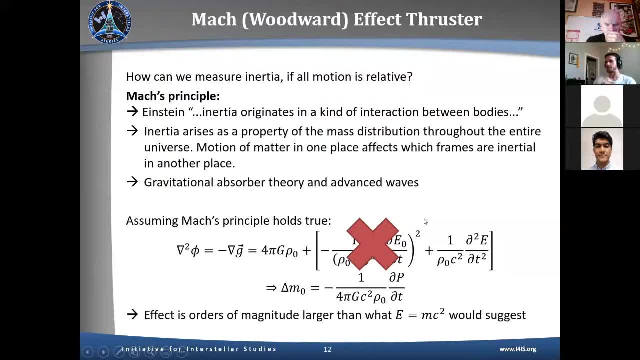 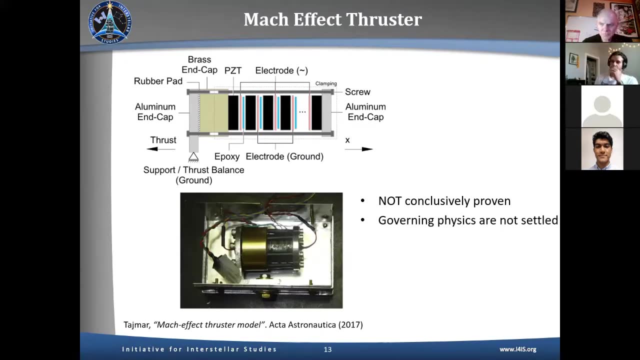 uh, the very familiar e equals mc squared, would suggest. and this is exactly what mark effect thrusters are trying to use. they're trying to use this effect, um, by combining a reaction mass with a piezoelectric actuator and a moving mass to rectify the sinusoidal effect into a directed 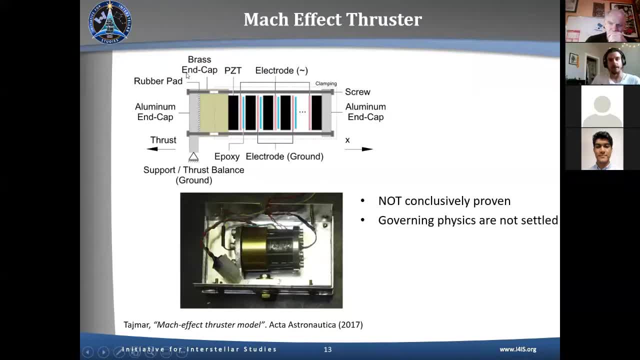 thrust. so here on the top you see a nice little uh sketch of what this would look like. so you have the pct elements, you have the electrodes. in between, you have a reaction mass that is mounted here and a mass that is free, and if you set this up correctly, the idea is that 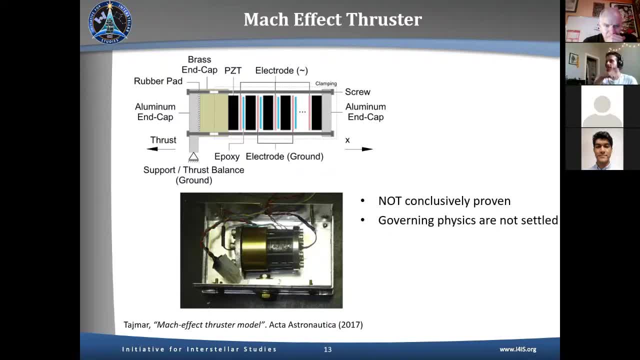 you can rectify this, uh, this alternating thrust into a directed thrust? um, this is a very interesting idea because it would enable propellantless propulsion, since all you need is an electric generator on board of your spaceship and this kind of device. but- and it has been tested quite a bit with different results, so it's not conclusively. 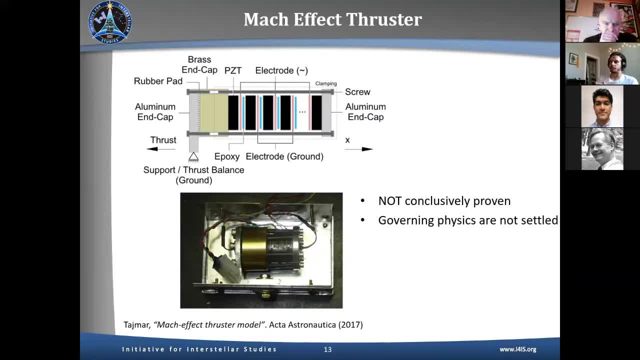 proven that it actually works and the governing physics is not entirely settled, so there's a lot of discussion going on about this. uh, there's further tests currently um financed by naiuk, if i'm not mistaken, uh, the nasa innovative advanced concepts program. so there might be some interesting results coming out of that in the future and if this works of 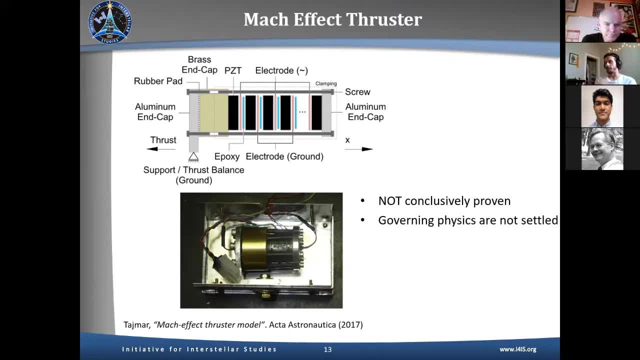 course. then we'll see how this works and we'll see how it goes on the next slide, And this would also indicate that the underlying physics might be correct, which has huge implications for a fundamental understanding of the universe And give you an idea of why this propellant that spaceflight is actually such a big deal. 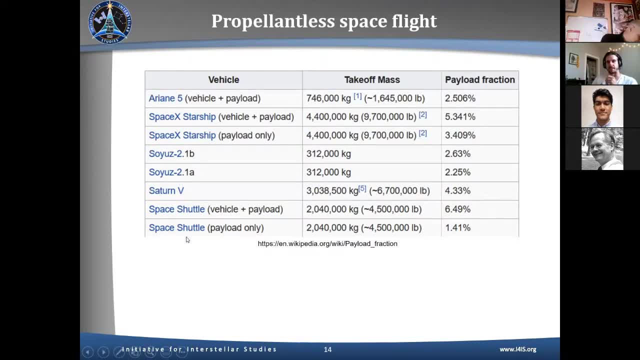 If you look at the different space vehicles that we're using or that we have used, you look at the takeoff mass, which goes into the millions of kilograms in some cases, And you look at their payload fraction. So a lot of the you can say 95% of the spaceship or 92% of the spaceship is propellant. 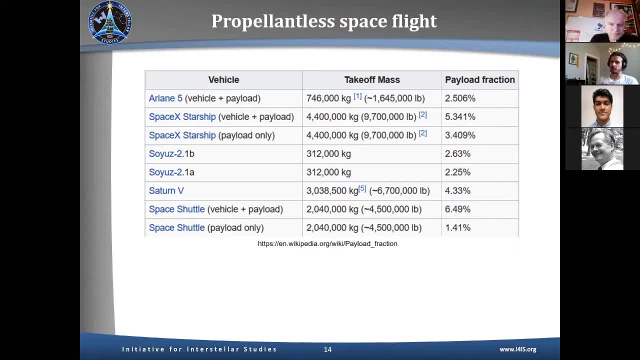 So if we can come up with a device that allows us to perform propellantless propulsion, this would be a huge deal, Because we could go much further with much smaller spacecraft. Or we can use the mass for life support systems- radiation shielding. 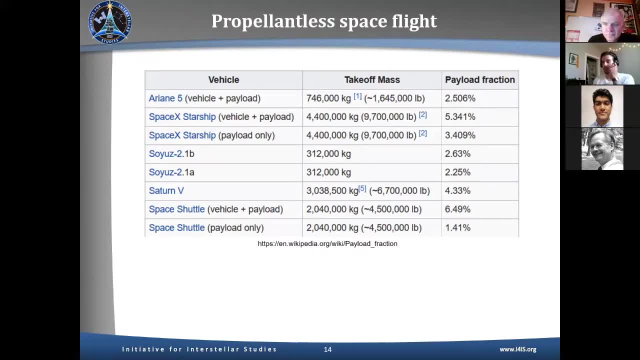 Or just for more payload. So this would be a huge deal if it actually works out. Of course, this kind of technology is, in a sense, well, it's not too crazy. with regard to the actual velocities that you can get, You're still moving at sub light speeds. 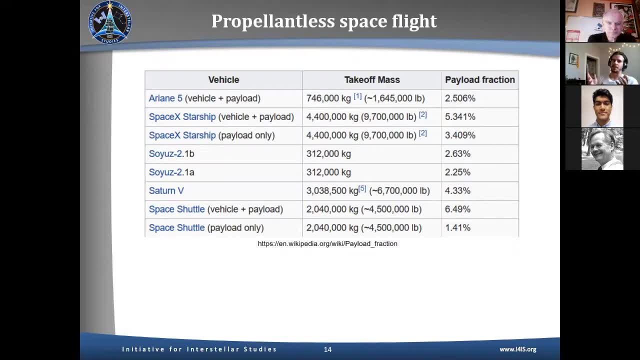 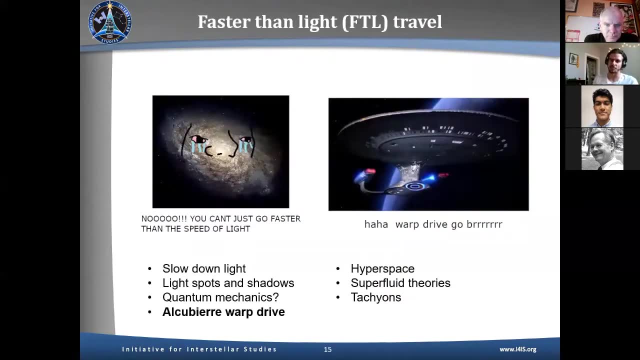 But one of the, I guess, most interesting implications of the theory of relativity is that there is actually ideas coming out of this to enable faster than light. So we know, on the one side we know that nothing should be able to go faster than the speed of light. 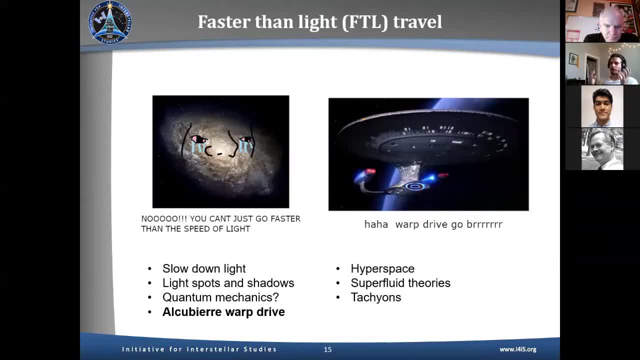 But we also have heard of probably a million concepts that propose exactly that. How can we manipulate the physics that we know to actually to still do it- to go around this limit of the speed of light? There's a couple different concepts that I've listed out here. 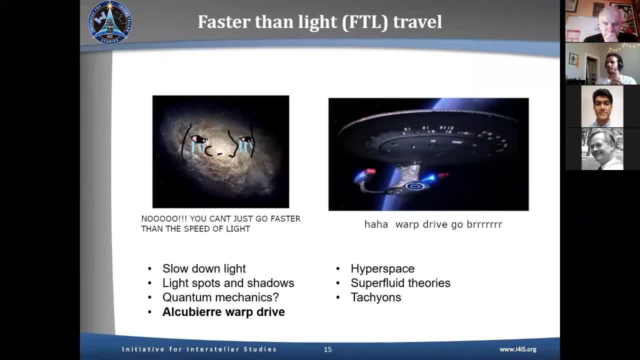 Like we could slow down the light And then just go back and then try to fly at the original light limit. It's kind of useless, because then we're not actually faster than the speed of light. Maybe there's something in quantum mechanics that would allow us to do this. 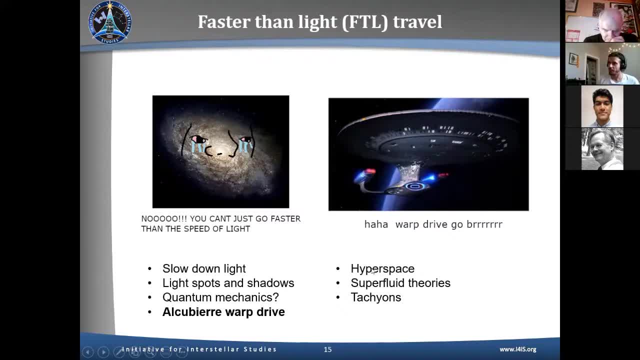 There's the idea of hyperspace travel, going to a higher dimension where, for a given distance, we travel much further in our three-dimensional space, And the one that has, I guess, garnered the most attention and that it seems at the moment the most realistic, although it's still very distant, is the Alcubierre warp drive. 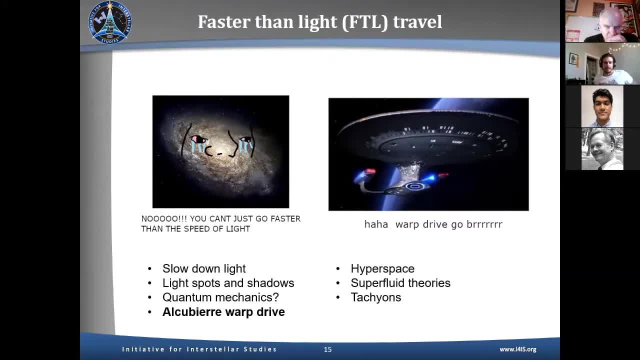 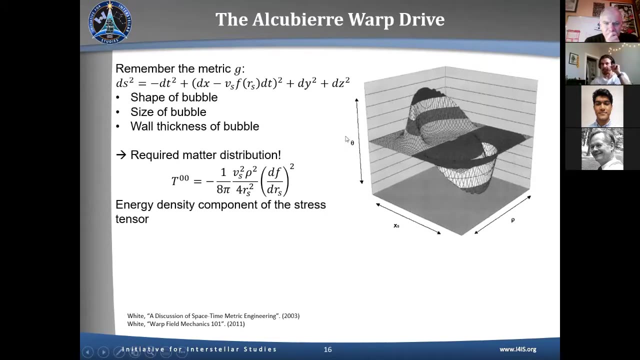 So I'm going to talk a little bit more about this, And this has also been mentioned in the last talk by Olivia, So I'm going to go a little bit more into the details of the physics. So the key to solving the Einstein equations and come up with something useful is to find the metric. 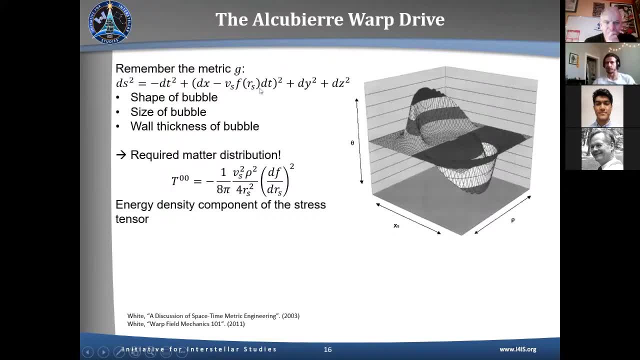 And this is notoriously difficult, but it has been done in a bunch of cases. Alcubierre came up with this idea of: well, if I can't go faster than the speed of light in vacuum, what if I just contract space, contract space-time in front of my ship and expand it in the back? 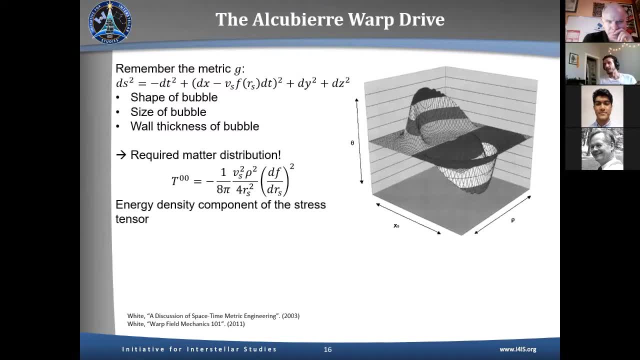 And so locally I'm never faster than the speed of light. But I can make this contraction so fast that I'm globally going faster than the speed of light. So you're not breaking any laws locally, but globally you would, And so you would. 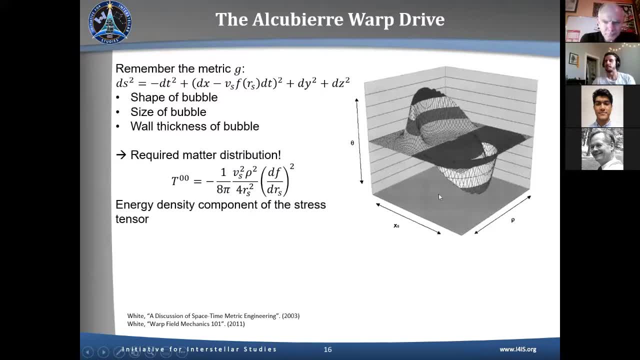 So you would create a warp bubble where this is kind of a hyperspace embedding diagram that shows what this would look like if you contract space-time in front of a spaceship and expand it behind it. And once you have this metric you can calculate. what kind of matter distribution do I need? 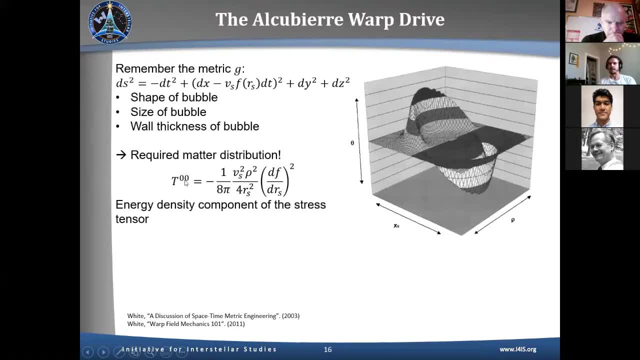 Do you remember this T00 that was in the energy mass tensor, And so you can calculate the matter distribution needed to get this kind of warp. It's very practical in a sense. The problem then arises from this negative sign, Because it tells you to create this kind of bubble you need a negative energy density or a negative mass. 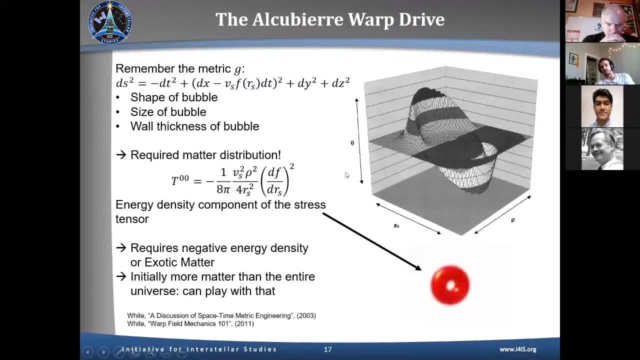 And this is also called exotic mass, And the initial results of Alcubierre indicated that you would need a mass, more mass, more negative mass than there is in the universe. So initially it's like, okay, this is interesting, but kind of useless. 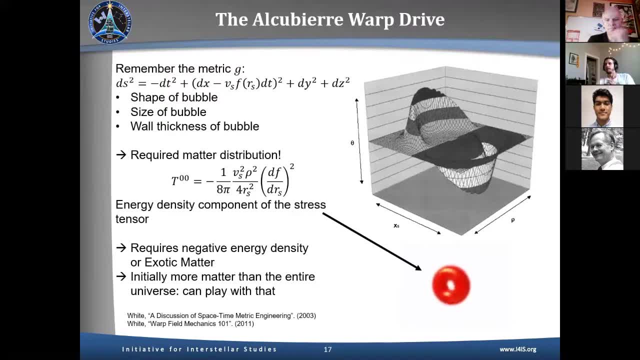 And people started to play with it a little bit more And they realized if they give the distribution of matter a certain shape like this kind of donut shape here, and then start pulsing the width of this donut, they can actually reduce the amount of matter needed to couple Jupiter masses. 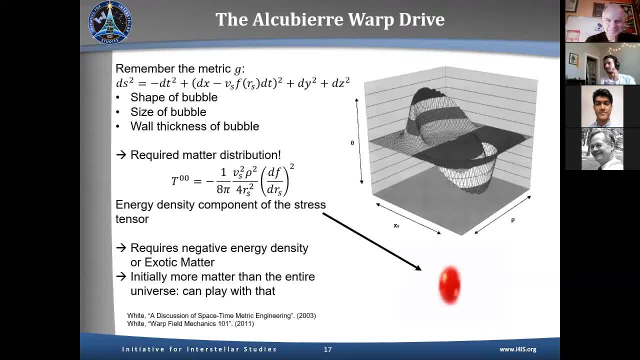 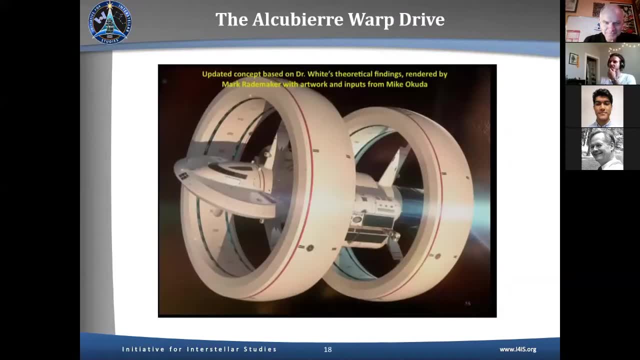 which is still outrageous, but compared to the entire mass in the universe, it's a. it's a nice improvement, And then they came up with these nice renderings. That's, of course, always very inspiring to look at, And I thought this is interesting because the shape of this spacecraft with these toroid structures is actually derived from the solutions of the Einstein field equation, where they say: we need to minimize the mass, we need a, we need a toroidal distribution of this negative energy or mass. 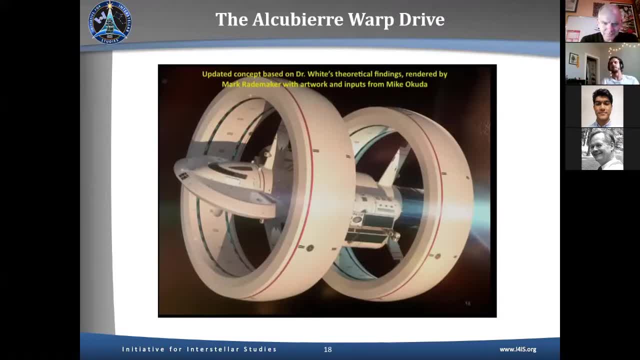 And we, hopefully, can pulse it in some way, And in that way we can create a spacecraft that is able of building such an Alcubierre warp bubble and going globally faster than the speed of light. Now, of course, you can already guess that this leads to some complications. 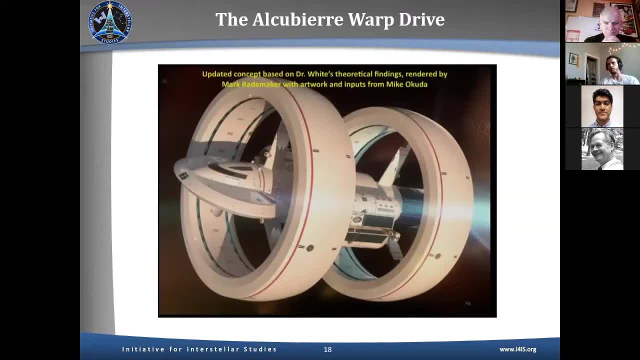 As we've seen in the space time diagram earlier, that when we move faster than the speed of light, we move into this non-defined space. where we are, there's causal disconnections, So cause and effect become a little wobbly and you're also disconnected from the other observers in the universe. and to illustrate this, 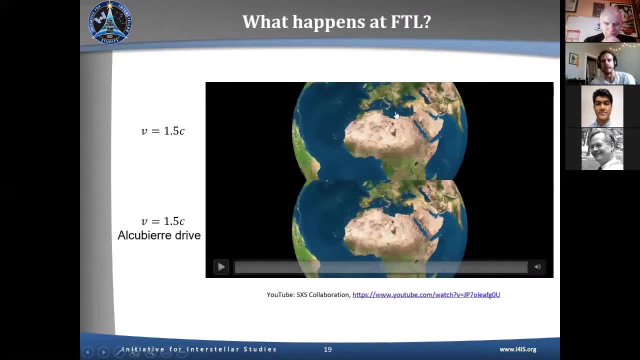 there's this nice simulation that I found on YouTube and on the top it just if you would be. let's say you're on the moon and you look at earth and you have a spaceship going by at 1.5 times the speed of light. that's on the top, and on the bottom you have the same spaceship, also again moving at 1.5 times the speed of light. 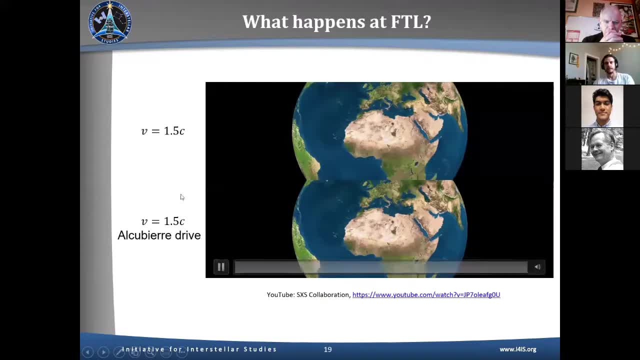 but this time with an Alcubierre warp drive And it's going to look weird. So you can see when the spaceship occurs on the top. going back a little bit, When it occurs on the top it's actually two spaceships that split up, heavily distorted. 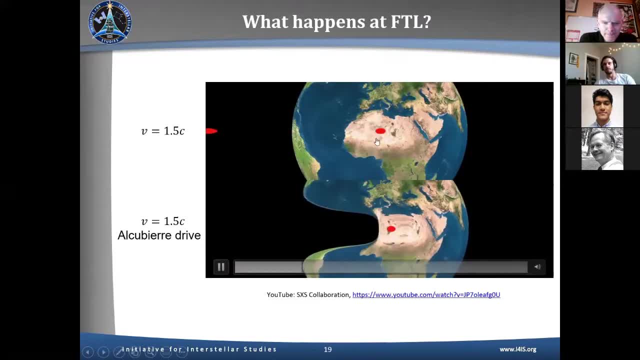 One moves to the left, one moves to the right, The one moving to the right becomes more circular And then, as it moves past the earth or out of our field of vision, it starts stretching again On the bottom, when we have, where we have, an Alcubierre warp drive with a warp bubble. 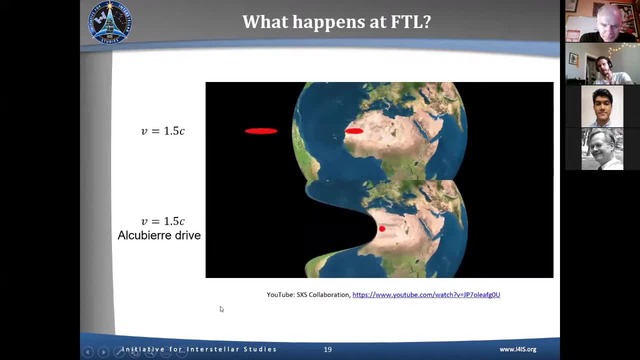 you see this weird visual distortion Again: the two spacecraft. the visual distortion persists, The spacecraft keeps moving until it goes towards the edge of our field of view And then, eventually, the visual distortion seems to disappear and it moves out of our field of vision. 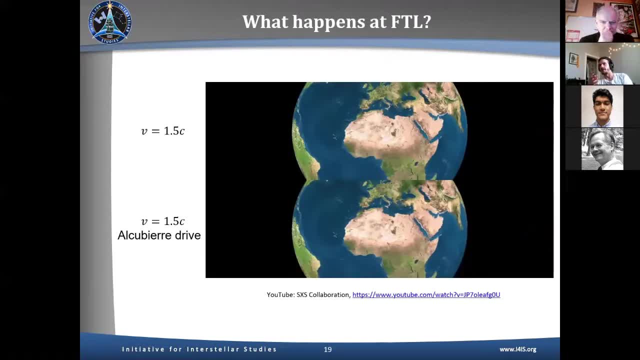 And the reason for this to occur is that, well, on the first, on the top, if we think back to our space-time diagrams, if we move faster than the speed of light, then the spacecraft is outracing its own photons, which means once its relative velocity to the observer is so low that we can actually see it. 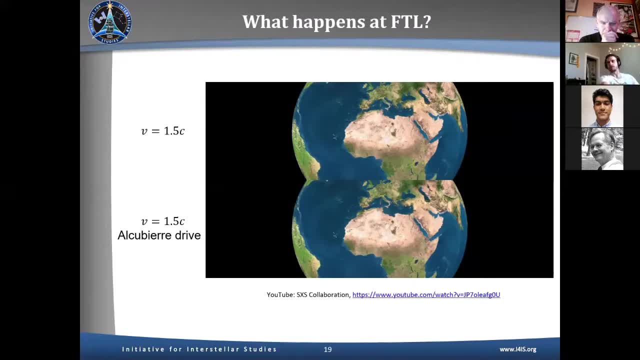 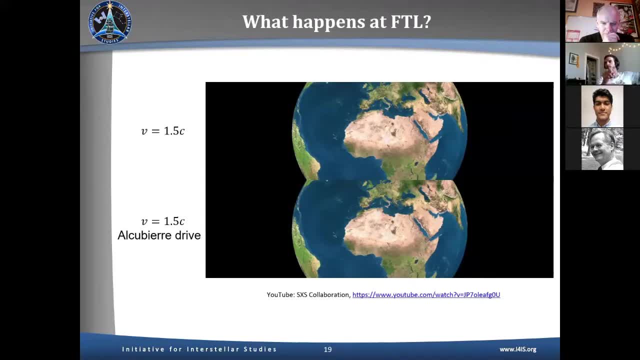 we will get photons from the spacecraft with a relative velocity below the spacecraft. we will get photons from the spacecraft. we will get photons from the spacecraft with a relative velocity below the spacecraft. we will get light speeds and we will get the old photons that the spacecraft outraced. 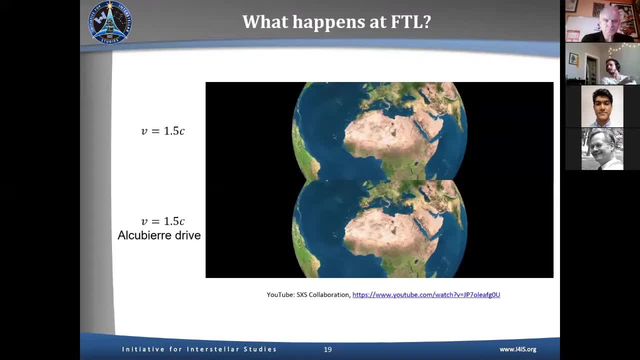 and we suddenly see two spacecrafts. We can still tell that the spacecraft is moving properly into the future, but it's a very like strange way of looking like. it's a very strange effect that occurs there. And then when we have the AlkaPey warp drive, 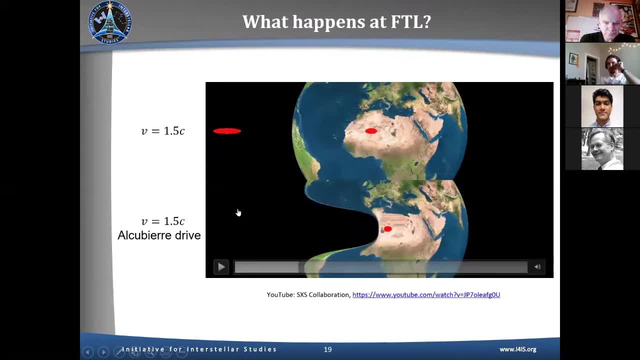 we get these additional distortions due to the gravitational lensing effect of the space-time distortion that we created in front and behind, due to the gravitational lensing effect of the space-time distortion that we created in front and behind the spacecraft. Everything else is the same as above, where the reason that we see initially 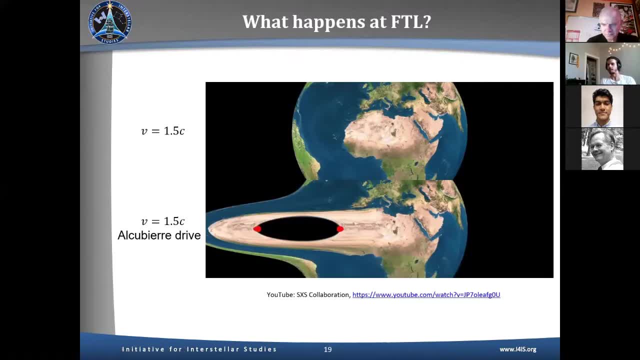 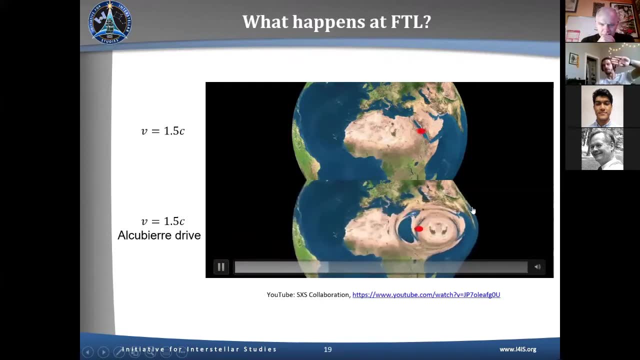 two spacecraft is that the spacecraft is outracing its own photons And then, as it's right in front of us, so its radial velocity is way below the speed of light. but then as it's moving out of our field of view and its radial velocity starts increasing again towards the speed of light, 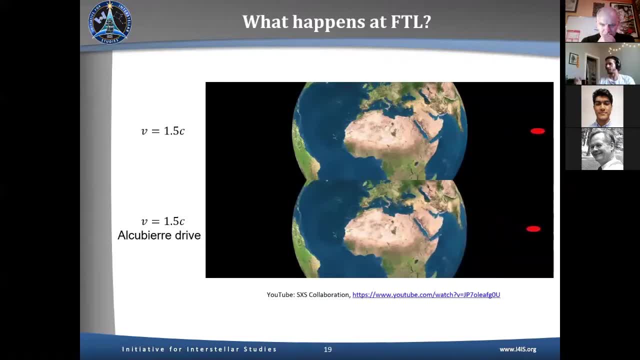 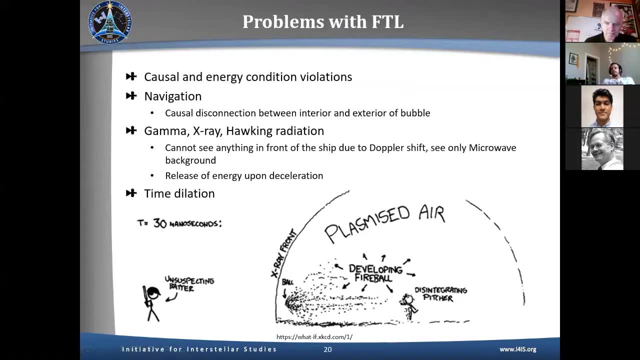 it starts stretching because of the space and time dilation effects that we talked about earlier. So we saw visually that there might be some issues with moving faster than the speed of light, even if we could do it, And there's more issues that are worth thinking about. So we have causal 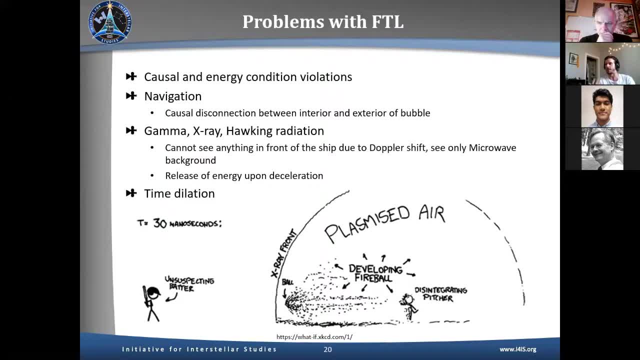 and energy condition violations. Energy condition is we need negative energy to do this. Causal violations because, technically, if you do this, because you're outracing your own photons, it would be possible for the spaceship image to arrive in the past, before it was actually launched, which should not be possible. It's kind. 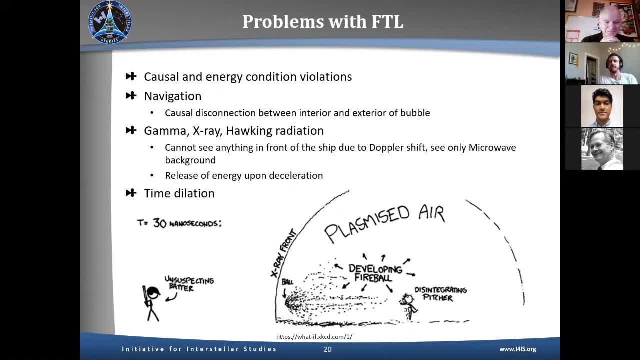 of mind-boggling, but this is what all of the physics implies. Then navigation of the spacecraft would be very difficult because you have a causal disconnection between interior and the exterior of the bubble. Nothing on the interior can reach the exterior And on the interior, 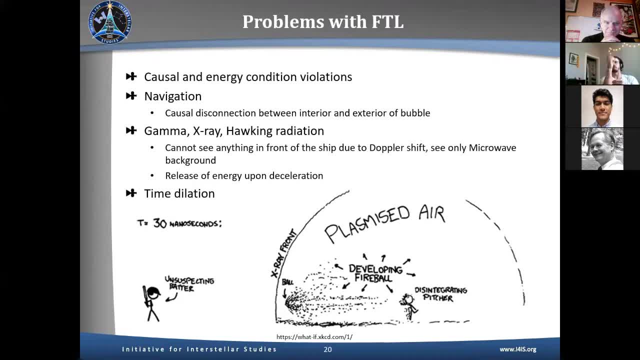 everything you look at, because you're moving faster than the speed of light. everything coming towards you is infinitely shifted into the UV, So it's becoming x-rays, gamma rays, And behind you everything is infinitely shifted into the infrared, So you cannot see anything there either. 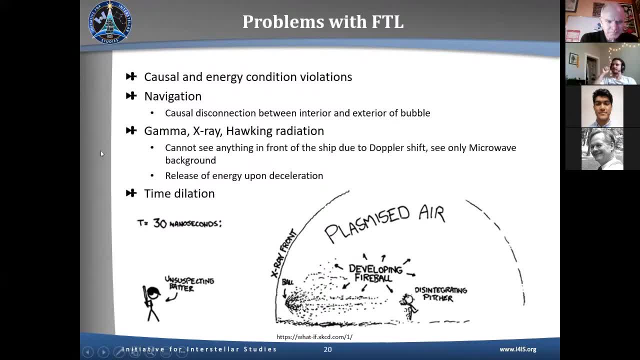 There's also the problem that once you actually hit the speed of light, there's the possibility of a very strong beam of Hawking radiation disintegrating you. So you're actually not going anywhere. So that would be a quantum effect preventing you from going. 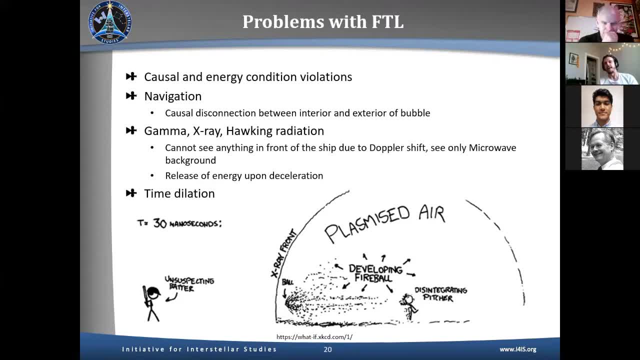 faster than the speed of light. We just don't know if that's going to happen. And then there's the possibility that once you decelerate, there is a release of a massive amount of energy in front of the ship which could disintegrate your target location. So you want to go to a nice tropical 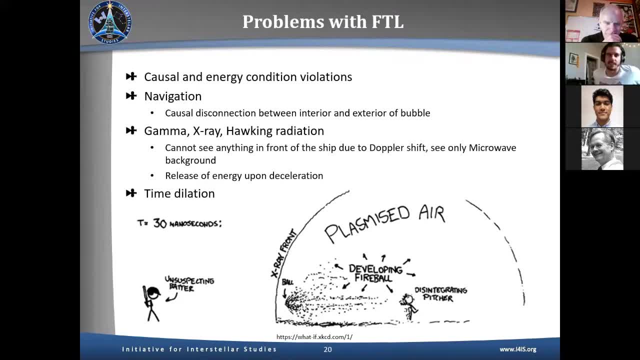 planet. You get there, disintegrate the planet. It's a little unlucky. You have to go somewhere else, maybe park parallel this time. And of course, you have time dilation, Where, even if you fly in this type of spacecraft for two years, by the time you reach your target. 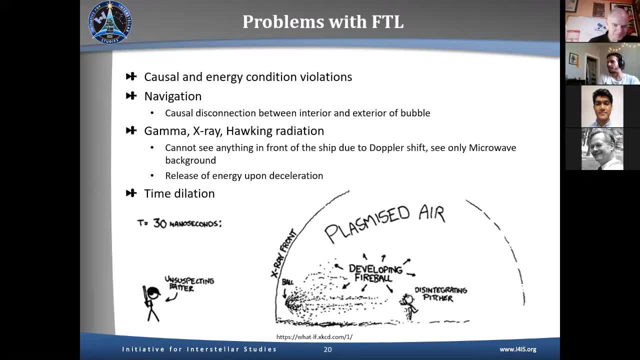 everybody you know back home would already be dead. I think that's a very kind of famous implication, but I wanted to just bring it up. So these are some very interesting things that can happen when you're trying to break the light barrier And with regard to producing negative 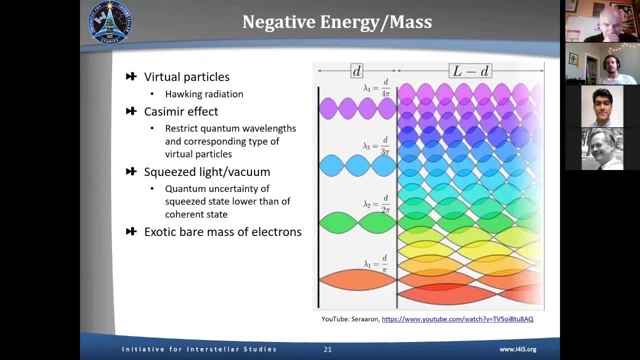 mass or energy. this is being actively discussed, if that's actually possible because it has been observed and there's some physics that in principle says it is possible in principle, We're just not sure if we've ever observed it. So one would be. the Hawking radiation: We know that the particle pairs 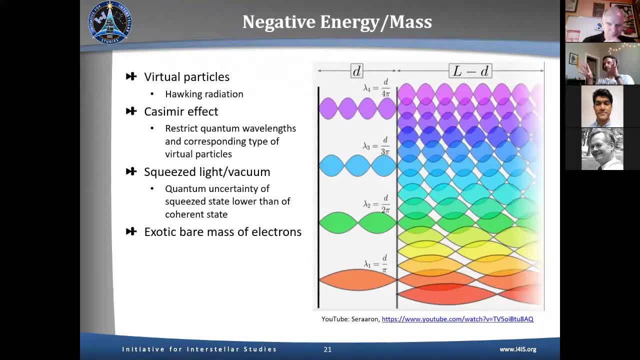 that are created on the edge of a black hole. one of them should be positive, one of them should be negative. The positive part is released- That's what we observe as Hawking radiation or would observe- And the part that stays is the negative part. So if we could somehow finagle that negative. 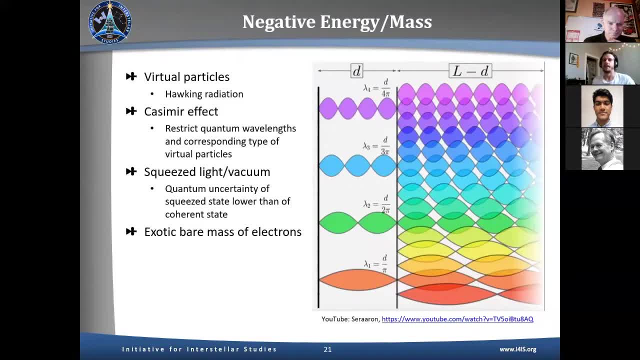 part out of the black hole, we would have negative mass or energy. Then there's the Casimir effect, which is illustrated here on the right, where you have two plates that are very, very close together, So you're restricting the wavelengths that are possible to exist. 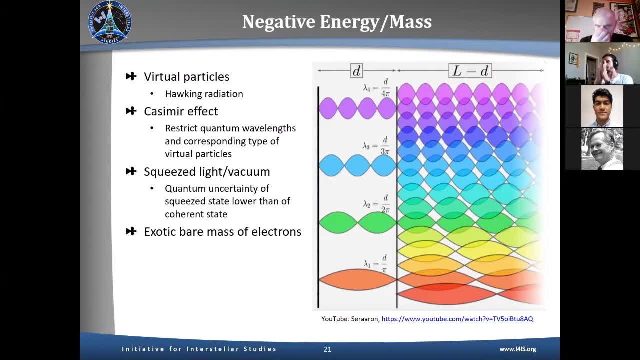 in between this space And due to this restriction you're creating a negative energy or negative energy density compared to the surrounding vacuum. So you can see, here on the right you have a much richer zoo of waves or of quantum fluctuations. here on the right in. 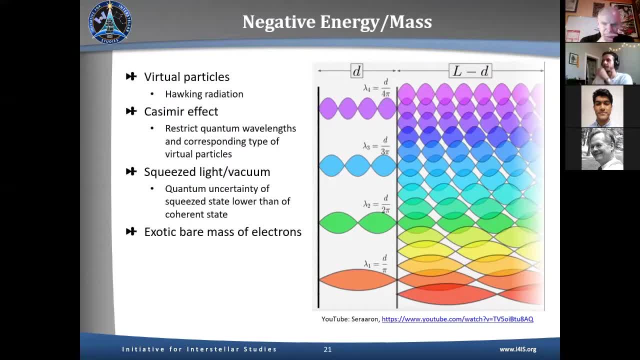 the vacuum, Whereas inside of the cavity you're restricted to waves that correspond to multiples of the length of this cavity, And that creates this negative energy relative to the surrounding vacuum which we might be able to utilize in this type of in a faster. 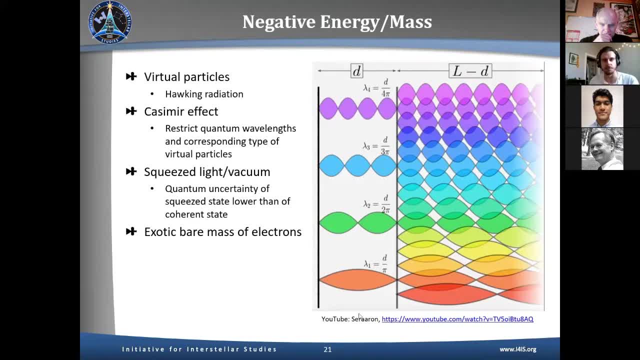 than light application. There's also a concept called squeezed light, where the quantum uncertainty of the squeezed state is lower than that of a coherent state. So relative to the coherent state, you're in a negative energy state And it's a little questionable if that is really giving us. 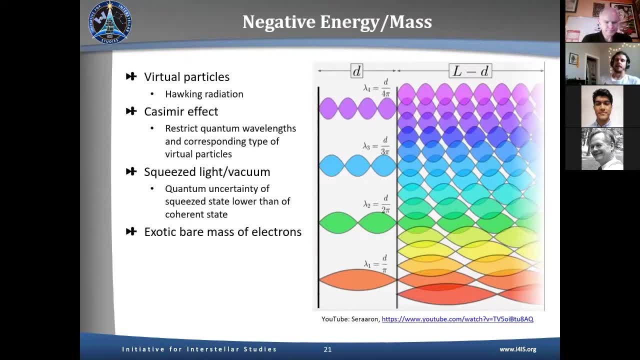 negative energy or mass in the way we would need it. And then finally, there's the idea that an exotic bare mass of electrons could give us negative mass. This has also been discussed by Woodward a lot And, yeah, it's speculative, but it's an idea, So I just wanted to put it out there. 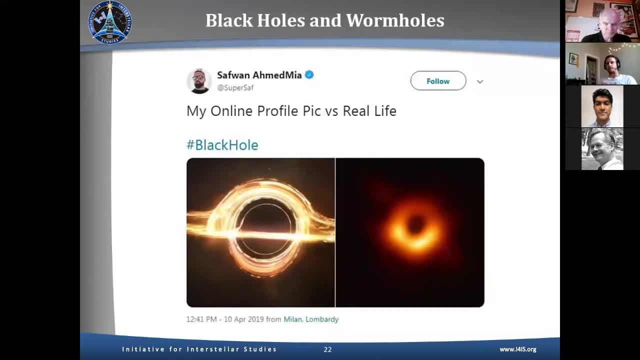 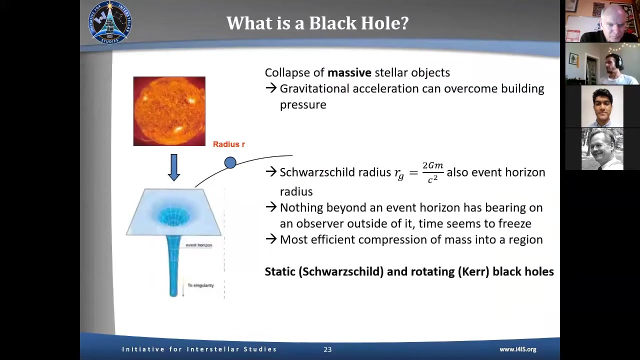 Now, instead of building our own space-time distortion machines, we can also think of maybe trying to utilize something that already occurs, naturally, in this case black holes. So a black hole just as a reminder is created when you have a collapse of a massive stellar. 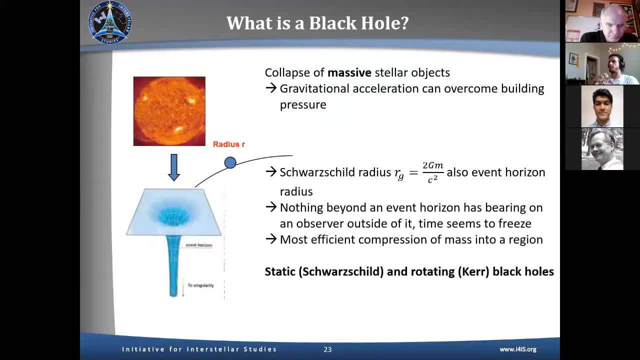 object And when you have a collapse of a massive stellar object, the gravitational pull becomes so strong that it overcomes the pressure as the stellar object collapses And eventually the gravitational or the space-time distortion created by this concentration of mass and energy becomes so strong that we create what we call a 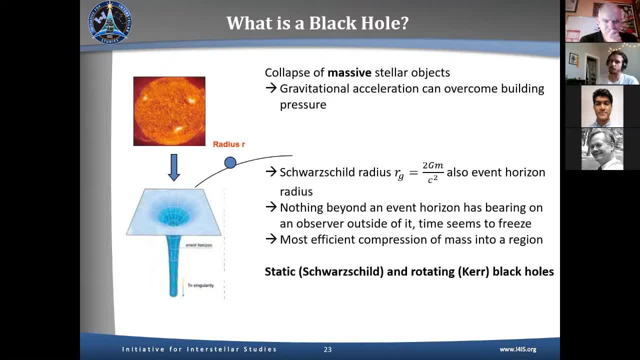 singularity, a point where the Einstein field equations break down And, as far as we know, nothing beyond a certain point around the black hole can have any bearing on the observer outside it. Time seems to freeze for an outside observer And, as far as we know, this is the most efficient compression of mass into a region that exists. 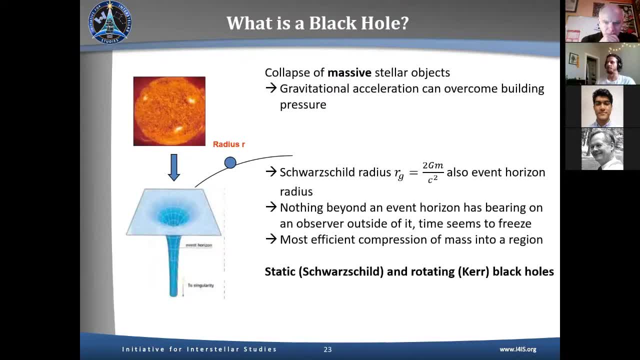 That seems maybe a little like an arbitrary point, but if you're interested in extracting energy out of something, it's actually very important, because then specific energy of something is of interest. There's a couple of different types of black holes And two of the 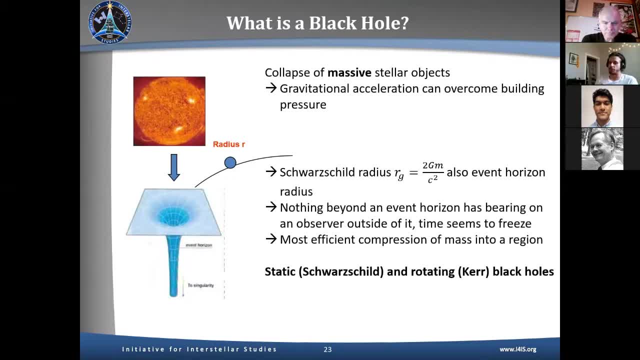 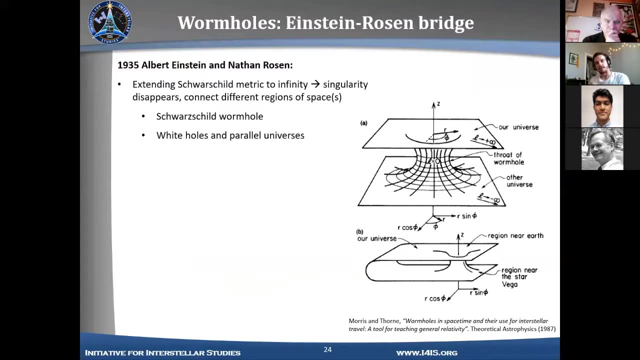 more important ones are static or Schwarzschild black holes and rotating or Kerr black holes. Schwarzschild and Kerr are the two people that found the solutions that describe these kinds of black holes to the Einstein field equations. Now, what Einstein and Rosen noticed? 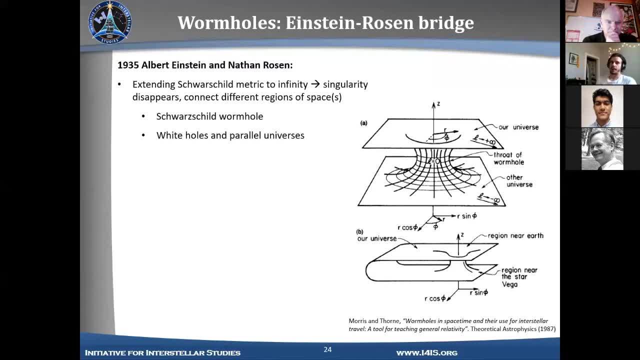 was. if they take the Schwarzschild metric for a static black hole and they just extend it to infinity to get rid of the singularity, then suddenly we are connecting two different regions of space and maybe even of different dimensions, And now what we call this often is a wormhole. 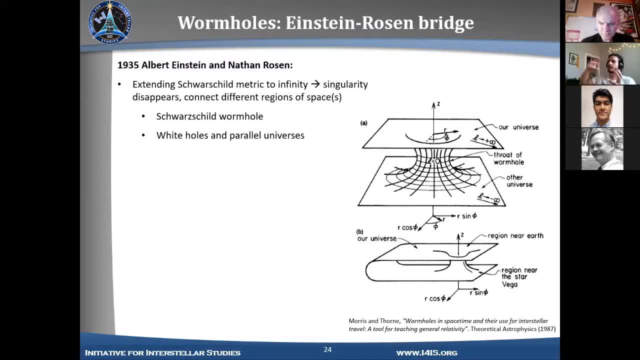 and we think of it as a shortcut through our universe. So this is illustrated in the bottom. If you have a two-dimensional sheet, this idea of folding it over and just poking a hole through it. so this is the idea of extending the Schwarzschild metric to infinity. get rid of the singularity. 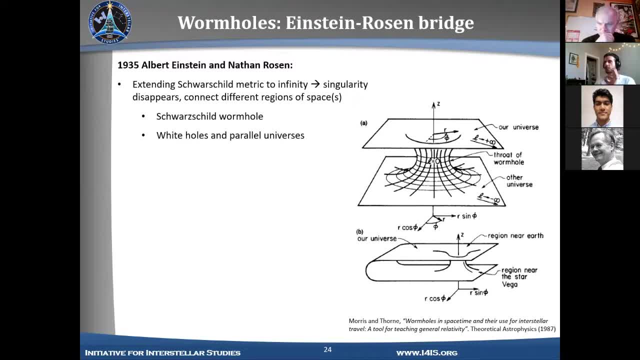 and you can travel a much shorter distance through the wormhole than you would if you would just stay in your regular space-time. Of course, it's not that easy. as you can probably imagine. If you want to actually travel through a wormhole, you would need to avoid the singularity that's. 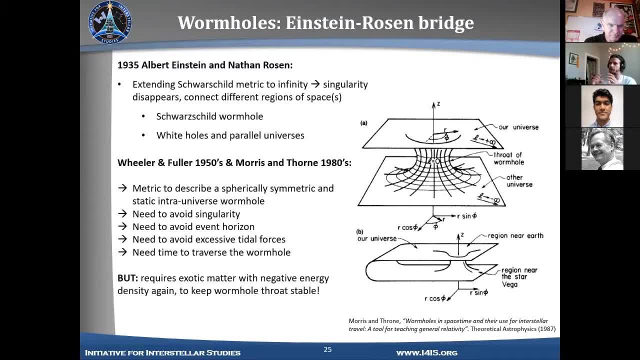 there and the strong tidal forces that are acting on the inside, You would need to avoid the event horizon and you would need time to traverse the wormhole, And one of the first things that they noticed when they looked at this closer is that a wormhole in principle. 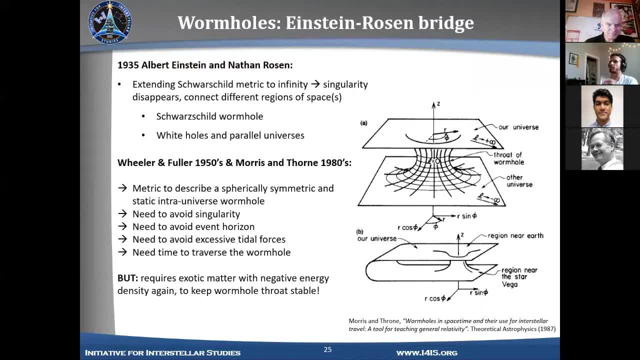 can form every time a black hole is created, but the pinch-off of the throat here is so fast that not even light can travel through it. And to stabilize this kind of wormhole again we would need a lot of exotic matter with negative energy density. so we're back to the same problem. 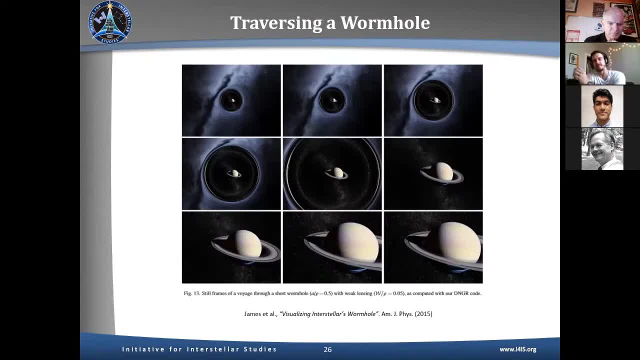 So showing you this because I thought it's kind of neat to illustrate what it looks like to go through a wormhole. So here you're on, let's say, our side of a wormhole. On the other side it's a different stellar system And you can. 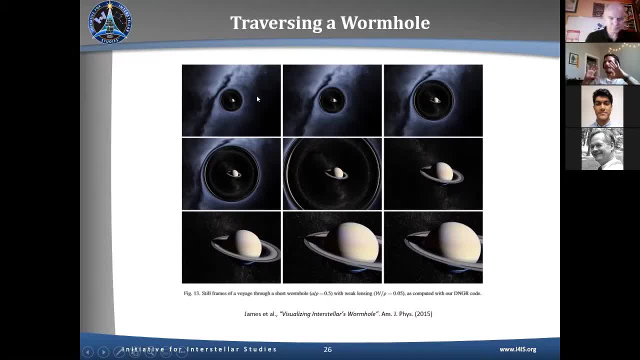 see. this distortion here is due to the space-time curvature at the mouth of the wormhole as it moves inward, so to say. But of course in a three-dimensional space it's a little hard to illustrate. And the interesting thing is that if you could make this work, you would 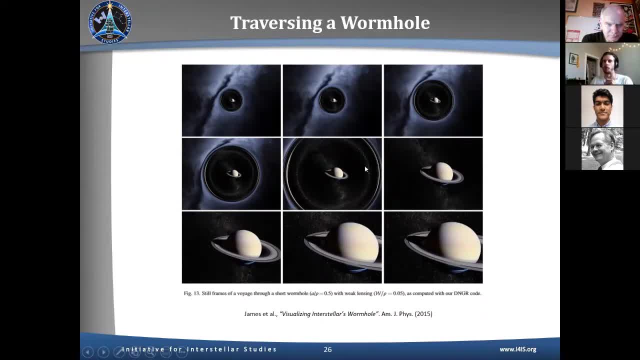 probably just go through. You come closer and closer to the wormhole you step through. there's nothing you would notice If there's no strong tidal forces and you can avoid the singularity. you just come out on the other side and hopefully save a lot of time to do that. 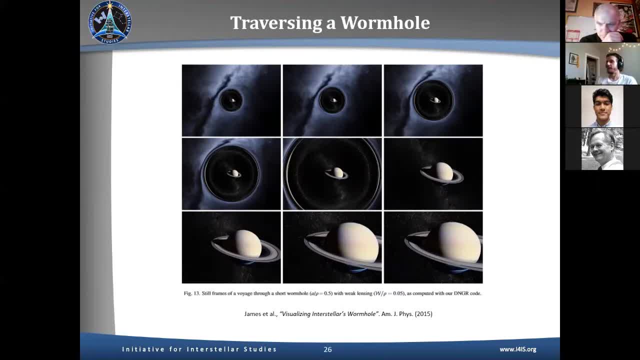 And another interesting implication of wormholes is that if something like this would be possible, you could also turn it into a time machine, And while this is a very interesting idea, this is also one of the main reasons why a lot of physicists think that, in the end, 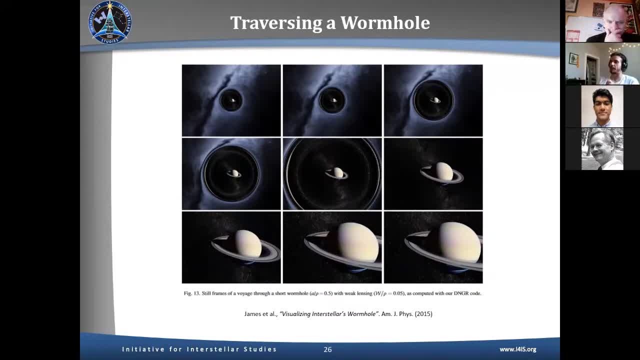 it's not going to be possible to construct something like this. Something in quantum mechanics is going to prevent us from building wormholes, whether that be a pileup of energy that destroys the black hole or the wormhole, or it could be that the singularity and the 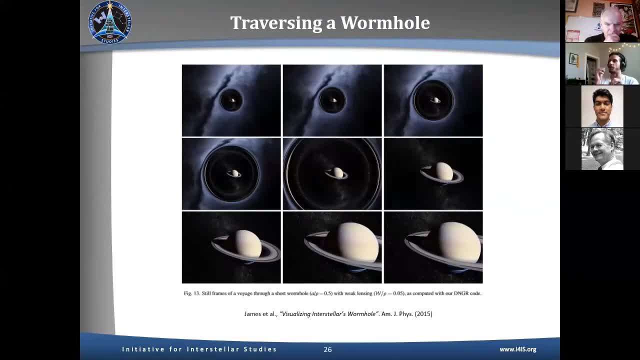 fluctuations that are associated with, such that they would always pinch off the wormhole. They think that something will prevent us from building this, But of course that doesn't stop people to think about it, because it's an absolutely fascinating prospect: exploring the edge of what we understand and maybe coming up with really far outlying. 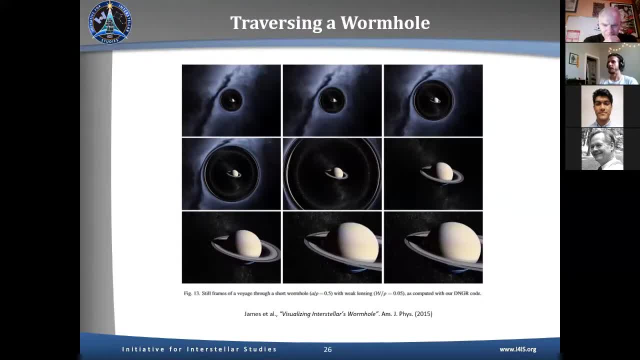 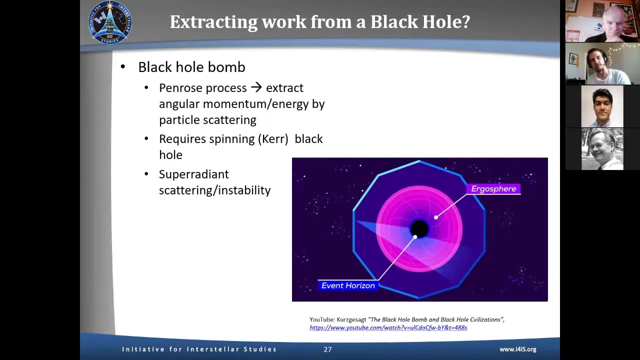 solutions to some of the propulsion issues that we have, and maybe issues of knowing the lottery numbers from last week and going back and putting them back in All right. So something that might be a little bit more practical but not by much is called a black hole bomb, because for something like this we would not have to build. 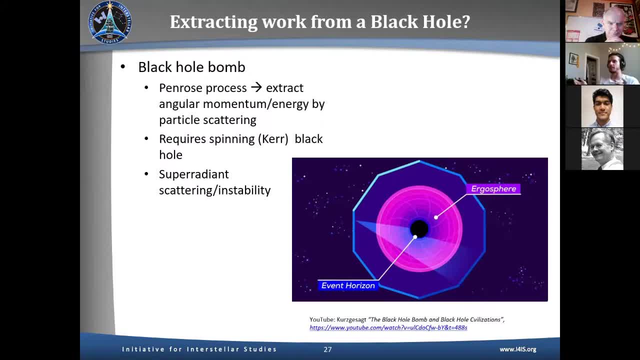 a wormhole. We would not have to change an existing black hole. All we would have to do is find the black hole that is spinning, And so if a black hole spins, it starts dragging space time around it. So you have an event horizon. It's illustrated down here. 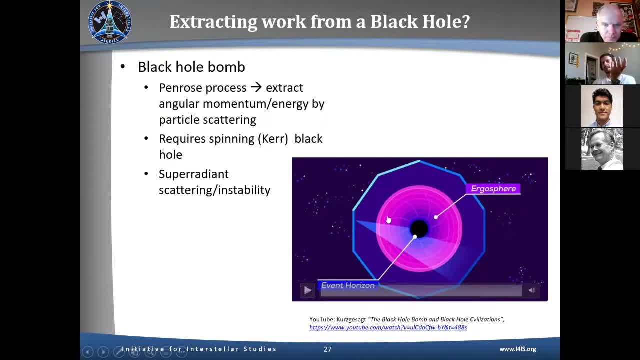 The black part event horizon is where nothing can escape. but around this event horizon you have swirling space time, and this is called the ergo sphere, And by something called the penrose process- after Penrose, who came up with this idea-. 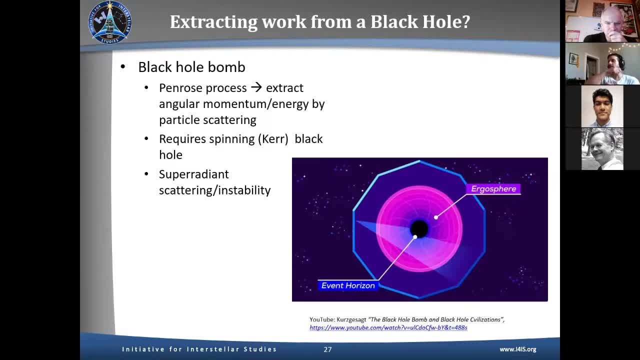 you can extract energy or work from this rotating part of space time. This is also called Super-radiant scattering, because you usually want to do this with a of light. illustrate this here, so you will construct a reflecting surface around the, around the black hole. you know this is sounds very simple so far. put a perfectly reflecting. 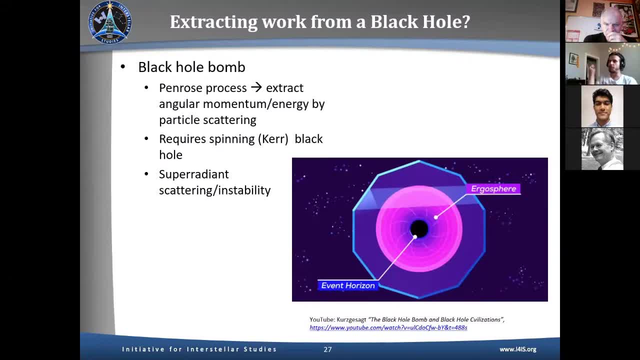 surface around an entire black hole and you will shoot a coherent beam of light into it, a laser, and of course you would have to hit the ergosphere so that the light always can just escape the black hole. it can never go into the event horizon and then it becomes, in principle, very similar. 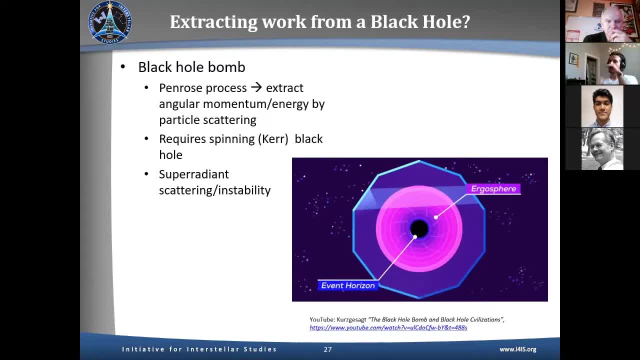 to a planetary slingshot or a gravity assist maneuver, where the spinning of the space time imports some of its energy on the light and the light carries it with it, and so, as the light is reflected and bounces around inside, it becomes more and more energetic. and well, it's called a. 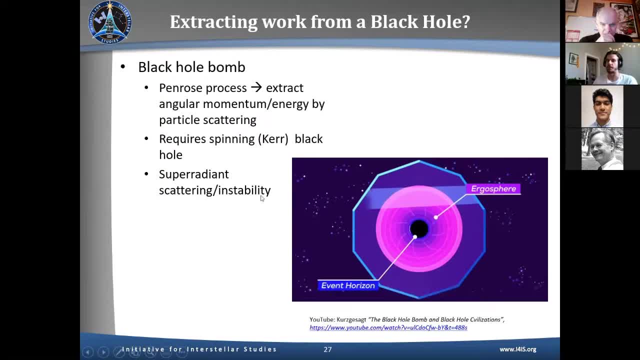 black hole bomb. you can do this until you hit the super radiate instability, and this would probably be one of the most devastating devices you could think of on a stellar level. or if we want to stick with the peaceful application, which is where i'm hoping this is going, then at some point you open the reflective enclosure and you 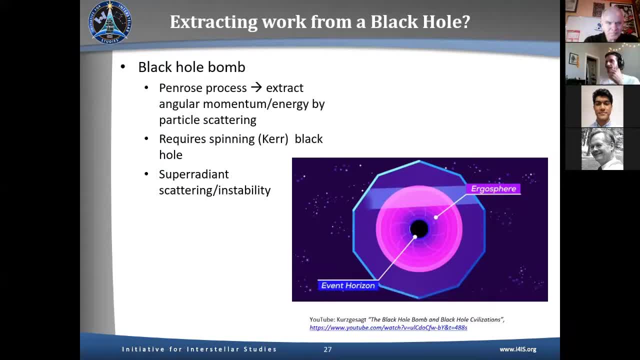 extract part of the scattered light that has now been energized by the swirling space time, and you use the additional energy from that to power any other devices that you might have. and in principle, uh, this goes beyond harvesting the energy of an entire star, so you might be. 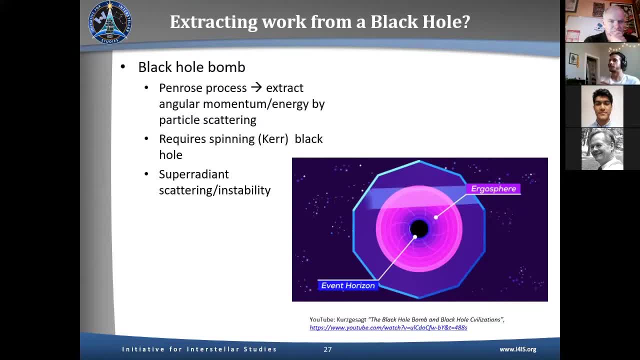 familiar with the idea of a dyson sphere or dyson dots. uh, uh, robert kennedy, if he's in the call where you try to extract the entire power of a star by building a sphere around it, um, this would be even more powerful, the powerful in the sense that you would have even more energy available for an even longer period of. 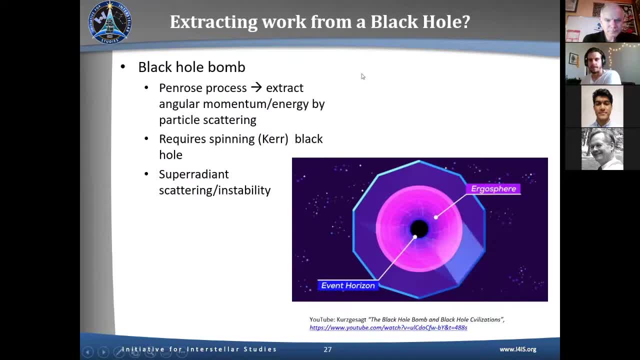 time. another way of extracting work from black hole would be to try and capture the hawking radiation. in that case, we would basically try to capture the energy in the same way we capture other times of radiation through antennas, resonators, uh converter cells, as in the case of. 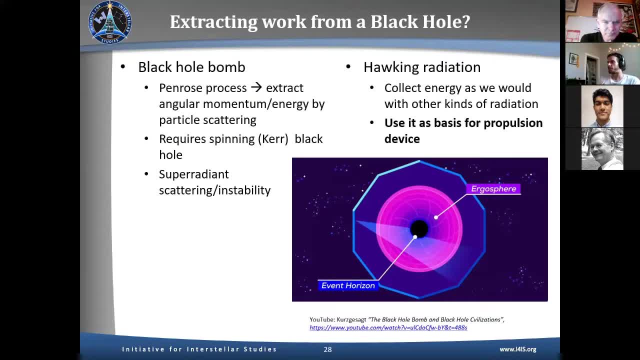 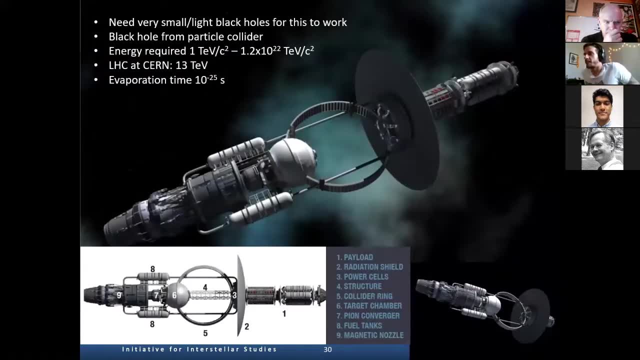 solar radiation and you could use that as a base for the implanting of black holes. if you have a scenario like that, you would always do that to capture the energy of a ball of light and you could basis for propulsion devices. actually, a couple years ago, um, uh, i4s came up with a concept like 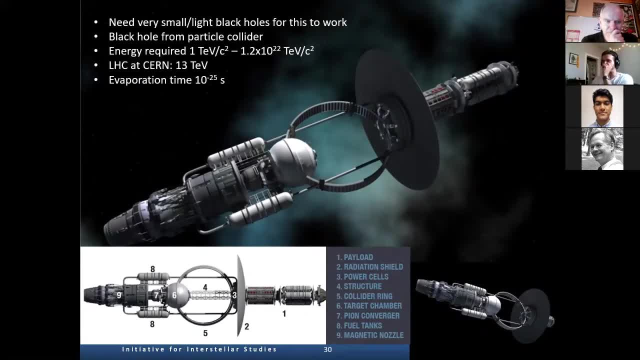 this, uh, where the idea was to create very, very, very small black holes in a particle collider that's shown here as a ring and then use the hawking radiation from those tiny black holes as they evaporate to power a starship. now there's a lot of problems there with quantum mechanics. 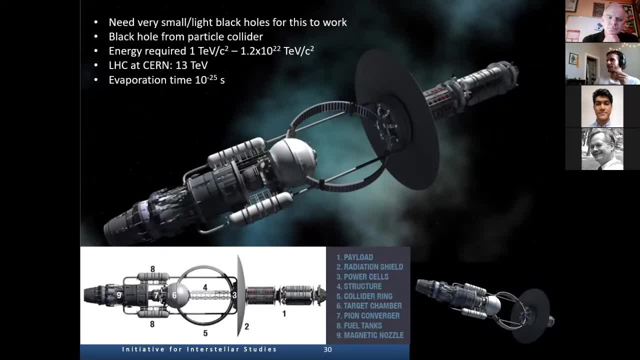 because when you go down to these kind of time scales here, uh, and the required energies needed to do something like that, uh, then it's not really clear if we would get even a black hole, if this would even be possible. but again, it's an interesting idea and an interesting concept. 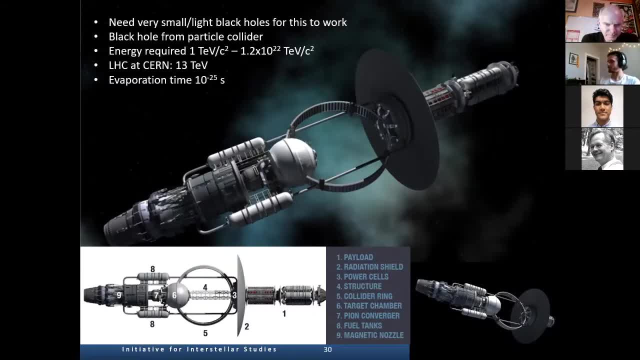 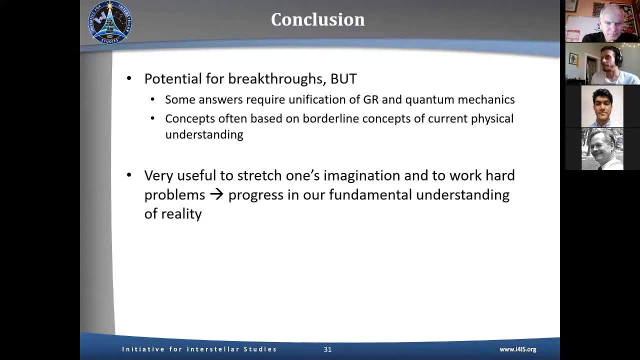 to try and push what we know about the physical world and uh yeah, i just want to leave you with these conclusions that the? um, the theory of relativity, or our knowledge of unified space-time, um has it has taught us a lot about the universe. um, there's a lot of potential for breakthroughs still, because some parts of the connection 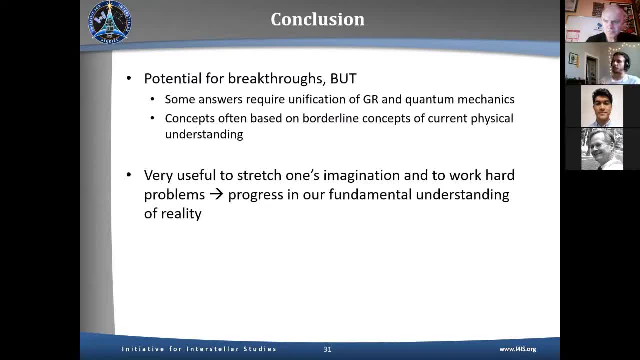 between relativity and quantum mechanics or the origin of inertia is not clear, and there might be a lot that's coming out of that. um, but you have to be careful with concepts presented to you, because a lot of them suffer exactly from the same issues that the underlying physics is not. 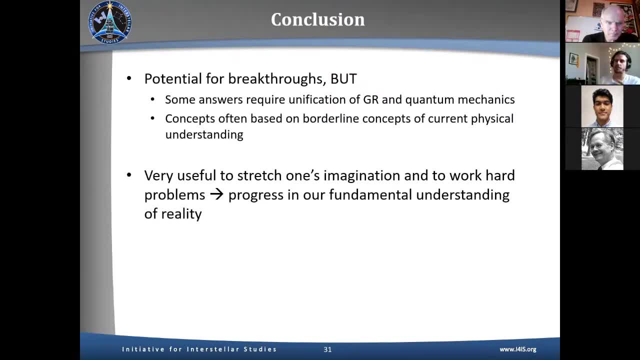 well understood that they rest on a very specific interpretation of the physics, or that sometimes it's wishful thinking and that some of the numbers just don't work out. but again, it's very useful to stretch your imagination, imagination and try it, and come up with engineering solutions on the edge of our fundamental understanding. and yeah, i hope that. 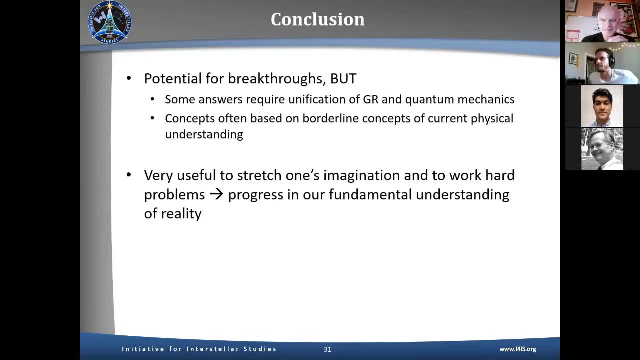 we have a little bit of a discussion about this now. okay, thank you very much, dan. that's a excellent whiz through. you're very prompt. that's brilliant. um, i'll just mention everyone. if anyone's wondering, we've got time for questions and answers, but dan does have to leave at the top of the hour. he's in texas at the moment, got a dash off to his lab. 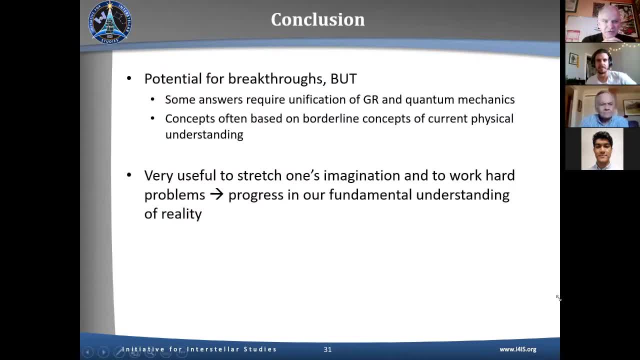 to sort things out there, but you can take questions for the next 10 or minutes or so, if if anyone from the floor has got questions- i see there's a couple in the chat, dan, i don't know if you can get them if you saw that. no, i didn't. there's one from patrick, one from patrick asking that that slide. 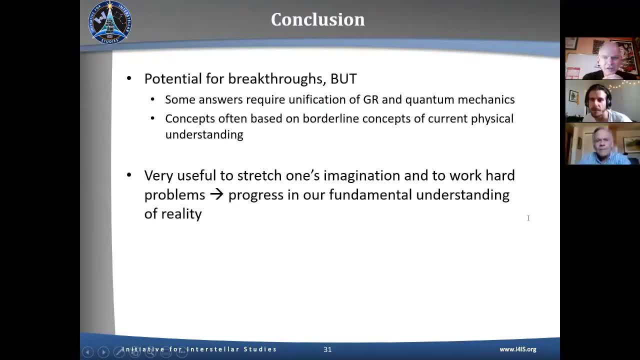 with the 1.5 c spacecraft going past earth. whether that's just a purely a visual effect, um, it is primarily a visual effect, uh, but if you would get caught in the too close to the bubble, where you have strong tidal forces, then of course that would be an. 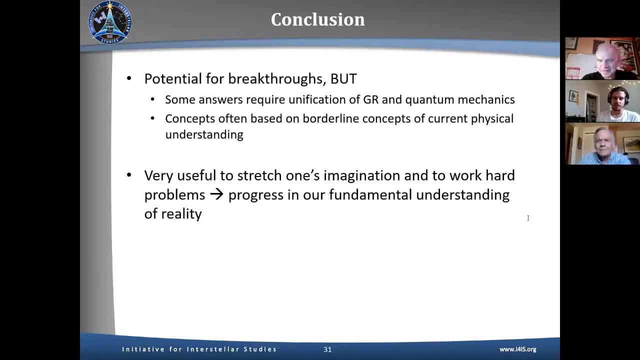 issue for you. um, so there is a the danger of physical damage if you would get too close and, of course, again once the spaceship decelerates, there's a chance of a massive energy blast being released from the uh warp bubble disintegrating and that also could cause real physical damage. 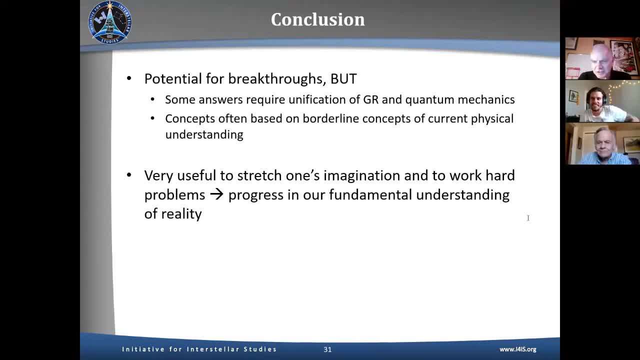 okay, i think that left in the chat also mentioned that there'd be. uh, you know, obviously if you move too close to the earth, there would be likely be a lot of energy blasts that would be damaged. that's what you're suggesting. so the huge gravitational force, yes, yeah, they would be. 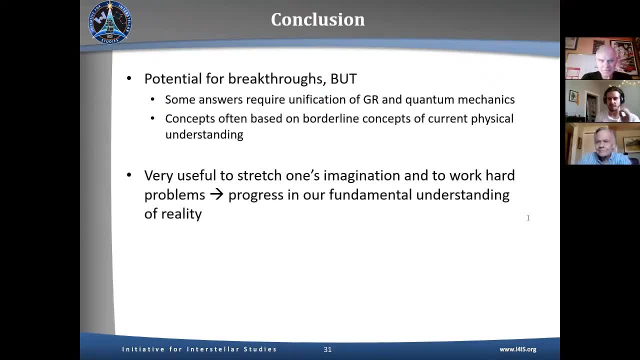 highly localized, so you can localize these strong effects very, very much. but, um, yeah, it is an issue. another reason, um, any, oh, i think you may have answered that one. how i read through that, it's about uh using hawking radiation. oh, yeah, so this is really interesting. yeah, so, uh, recently there's 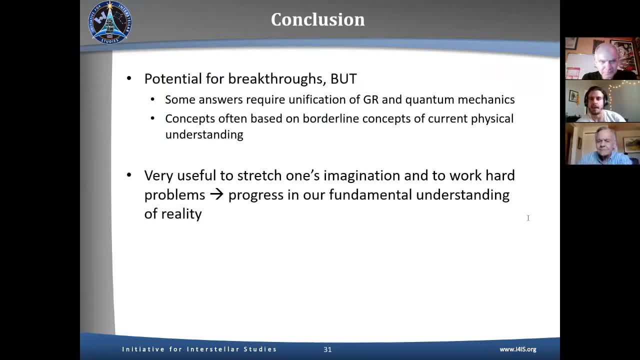 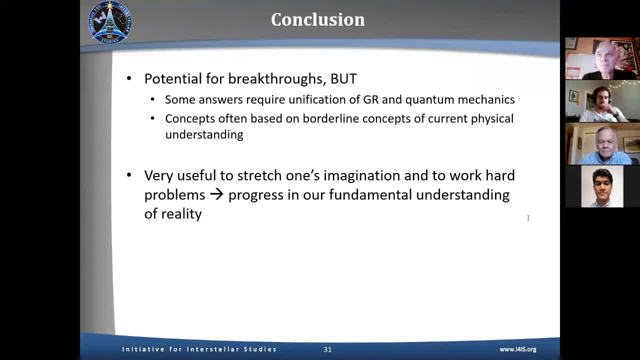 uh, using fluid dynamics, using optical mechanisms, even with acoustic devices, to build something that resembles black holes in its properties. um, so i'm very glad that was brought up. you should definitely look into this because this is something we can build in labs and investigate- and i have not read that paper but i definitely will because those uh analog. 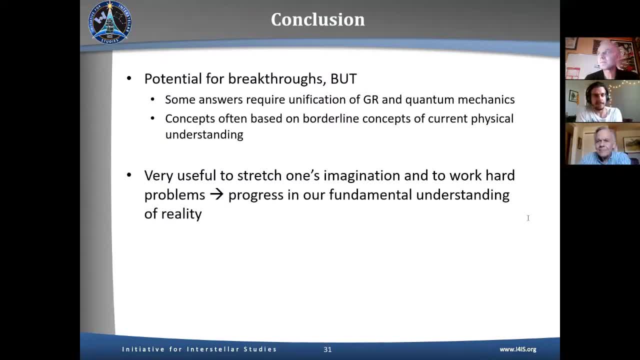 black holes. uh, they potentially allow us to investigate the nature of those virtual particles particles better, and if we can manipulate this in any way, then, yes, we might be able to extract very exotic properties out of that. okay, excellent, i see that. uh, john has got his hand up, so if you'd? 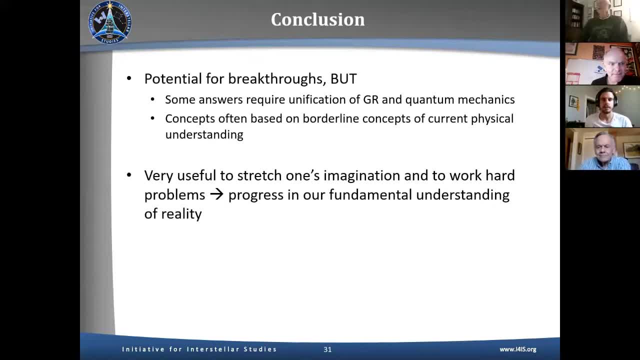 like to unmute yourself, john, and ask you a question. go ahead, hi dan. uh, the fun talk um ut physics back in the 80s, but um, so anyhow. yeah, my question um, it kind of relates to both the mock effect and the um alcubier, and in both of those, i mean, i've looked at them and i have a hard time kind of with. 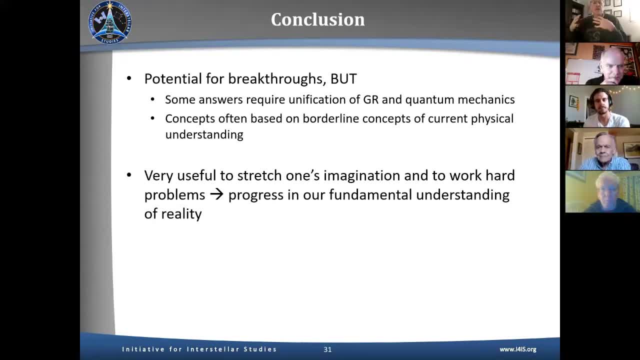 both of them and what it is is if you envision a um, a large volume with either alcubier or a mock effect in the center of it, asymptotically. i'm kind of flat in both of those cases and you know the mock effect, thruster. i kind of envision it as i've got a power supply and the 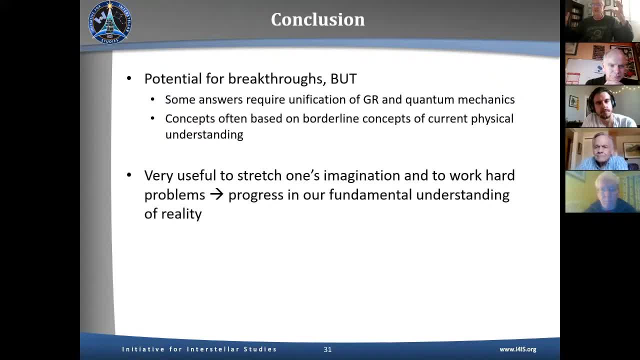 device and i could sort of think of it as you know: transfer of fluid or you know pumping something back and forth between the two um pieces, the power supply and the device. so asymptotically i don't see any mass change locally. on one side the mass is going up and down. so how that's going to move. 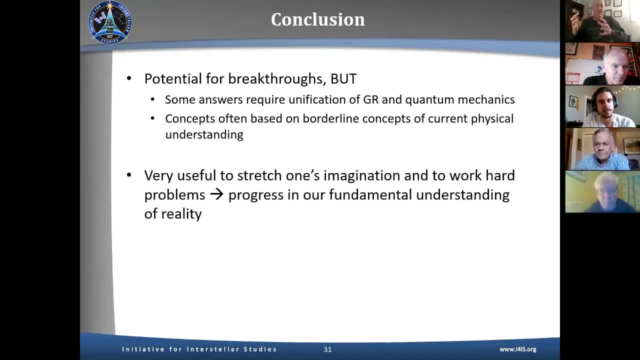 anywhere relative to the other side of the device and i'm kind of envisioning it as a power supply- distant stars I don't get, and Elcubier sort of similar in that. so I'm assembling the device and asymptotically the metric's flat you know, say I'm halfway between here and Alpha Centauri. 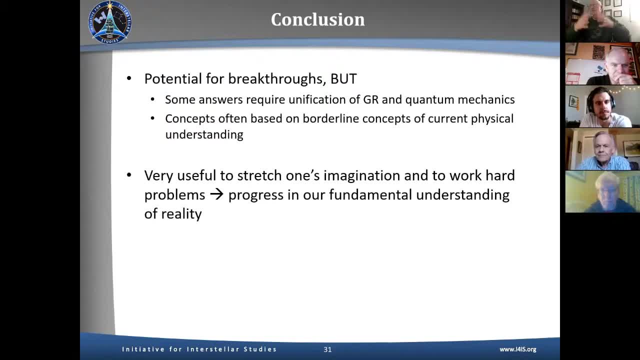 you turn that on, that ripple in the metric is still going to move like a gravity wave right and propagate at c, so I still don't see how you end up, you know, with moving from here to there at a um, any kind of um. you know superluminal velocity, so anyhow, yeah, so that's, those are very. 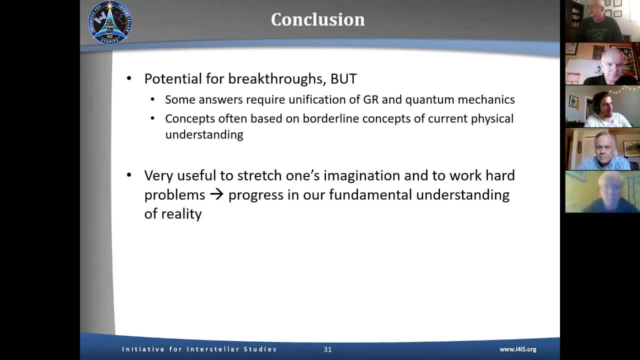 good points. uh, so to the mark effect, I can say something real quick. I think I forgot to say that. uh, specifically because it? uh, this is very much connected to the manipulation of inertia. these higher order terms only come in when something, when you have acceleration present. so the idea would be in this case that the power generator or your battery that is pumping energy, 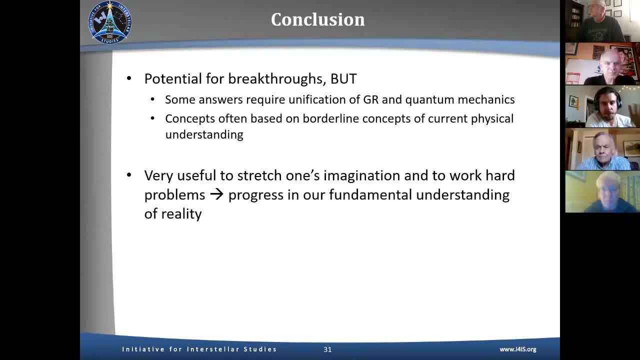 out, uh or in? is uh not affected by the mark effect, uh or woodward effect? because it's. it is not uh accelerated at the right phase relative to the change in the internal energy, whereas for the mark effect for the thruster device, um. that's why you have those p8. 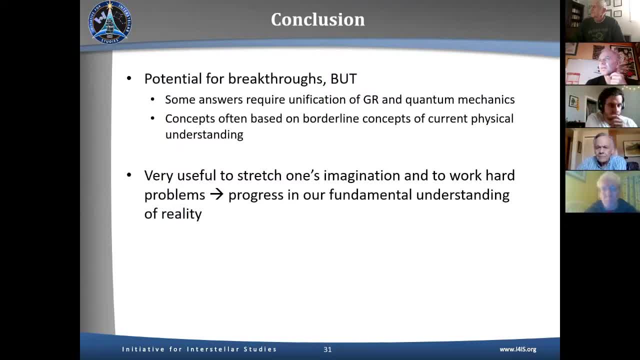 electrics that are expanding and contracting, you provide an acceleration at the in right, in the right phase with the change in internal energy to actually generate, um, the mass fluctuation. so that's how. I think that is the justification that is usually given for why it would work, and 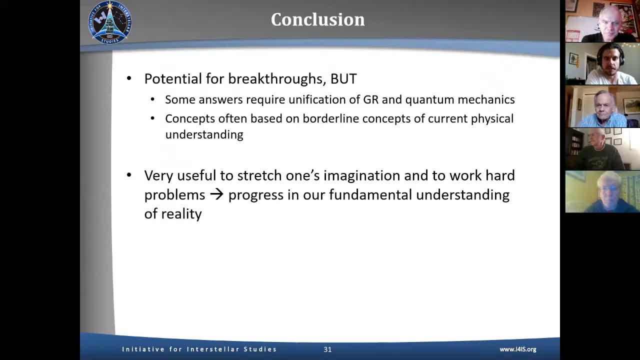 why it would not be nullified by a battery or the generator itself. um, for the Alcubierre drive. so, if I can get that correctly, uh, there is a difference between, uh, the ripple that you're creating for the Alcubierre bubble and a gravity wave, and that difference is what essentially 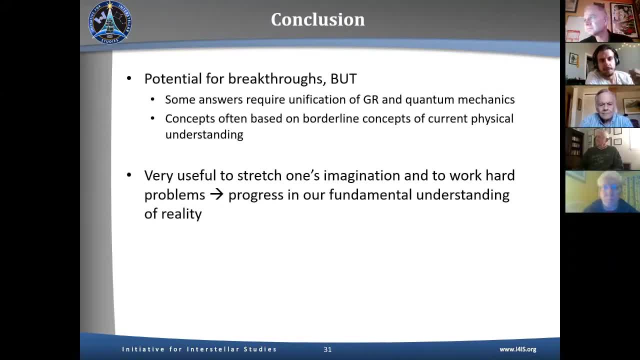 the idea is that you're moving. you're moving the ripple. yeah, so the gravitational wave is not a contraction and expansion of space-time, whereas the Alcubierre drive specifically does that to globally get you above the speed of light but locally keep you below it, so that, as as far as I understand, a gravitational wave is not a contraction. 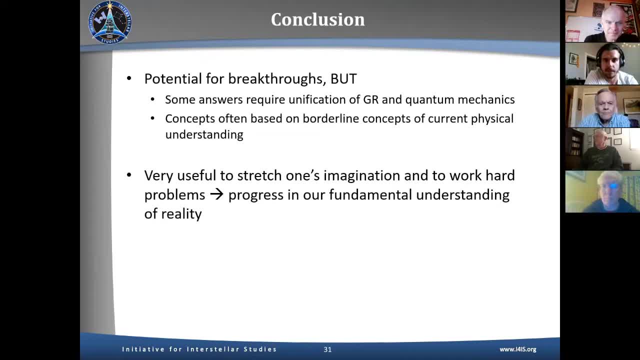 or expansion of space-time, in the same way that the um, uh, that, uh, sorry, Alcubierre bubble would be. but uh, you can, I mean I'm happy to if you have. uh, if you can extend on that a little bit more, I'm happy to talk about that. yeah, I mean, I mean I've- I've looked at it multiple times. 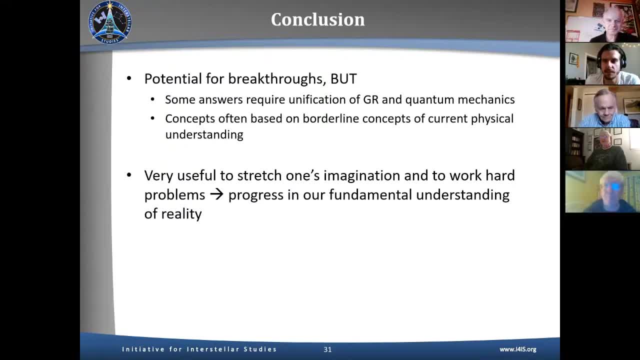 and I've just never been able to quite convince myself that there was anything that would, you know, come out faster than the speed of light. it always seemed to me like the argument that it was the expansion and contraction of space, like a hand-waving kind of an argument that I never really- uh, you know, was able to get to the. 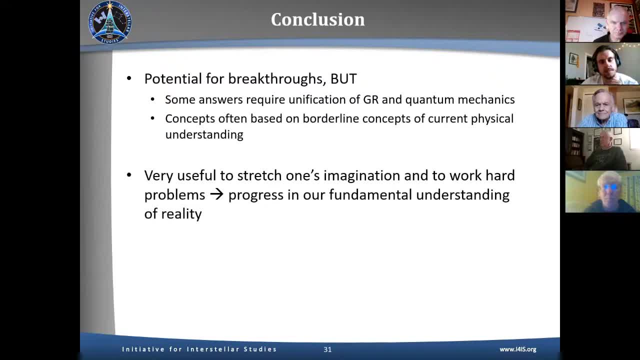 bottom of. I've crawled through Alcubierre's paper multiple times without really buying it and uh, and then people have kind of taken it and run with it, but at the very bottom of the argument it just doesn't seem to. you know, I just can't figure, you know, get my head around it in any way. 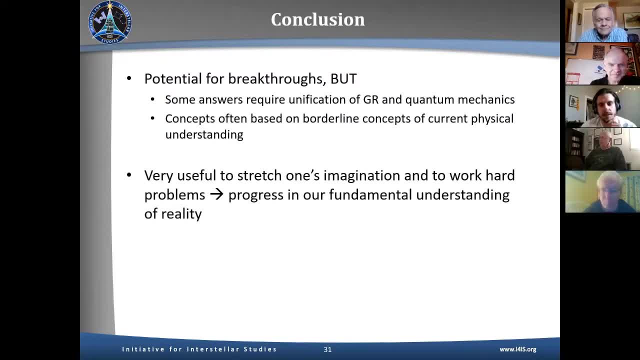 that. um, you know, I believe it's it. just, you know the, if you're perturbing the metric, I mean you first order. you know the, the linearized gravity that they use for the gravitational wave equations. um, you know, basically, start with here, here's a metric, here's deltas to the metric. 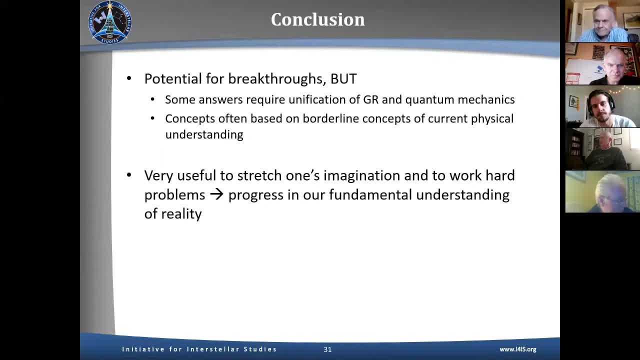 and you know they always come out propagating at c and and you know the art, you know the only only place anybody points to where things are moving faster than c is back during the inflationary stage of the um, early universe. and you know, and the underlying physics I think of what drives that inflation is still. 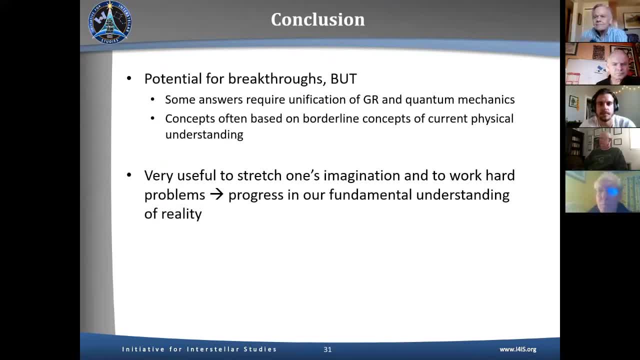 you know, an open question. they, I think, postulate uh, you know, fields that have, you know, never been observed, you know in an accelerator or anything like that. so you know it kind of fits the observation, but you know there hasn't been any kind of, um, you know, laboratory demonstration. 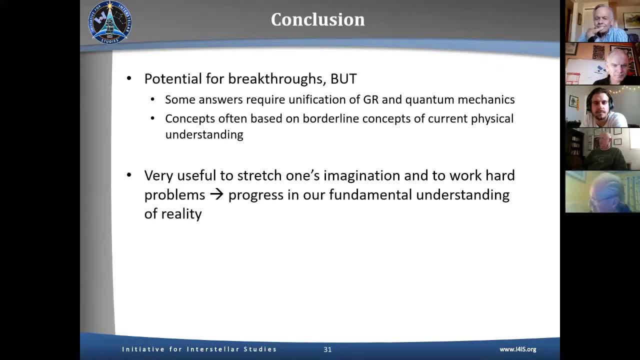 of the physics going on in the inflationary stage of the universe and I'm pretty pretty leery about turning inflation on somewhere locally in the universe and hoping that it I can turn it off again, uh, somewhat later. so, uh, yeah, that's a, that's a very good point, I mean. 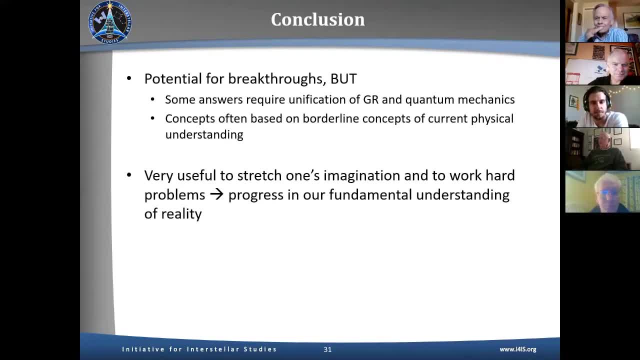 it goes exactly to this issue of uh, all of this some being somewhat speculative- um, I cannot give you a satisfying answer. this is something I would have to look at myself closer, but I'm going to keep that uh in mind for the future because it's a it's a very good question. 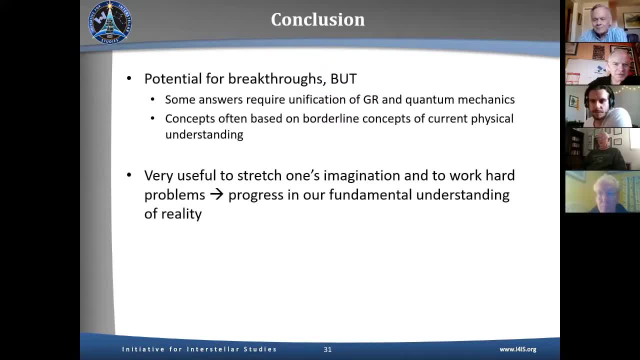 yeah, I mean, I think you know wormholes are a little bit more interesting and they certainly have some problems there. you know, lately in my um my day job is a- uh, an engineering physicist. but you know my spare time, you know, like to ponder the fundamentals in that and I've been poking 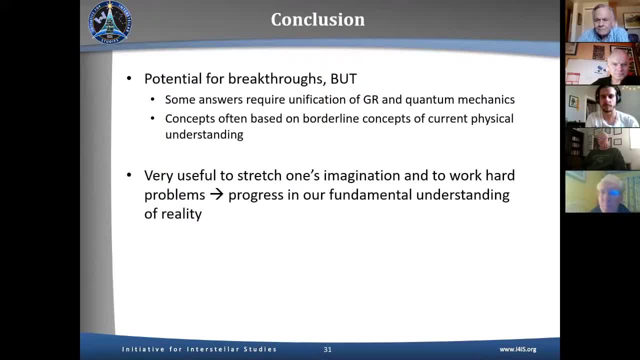 around at a paper by um Wheeler back in the early 60s where he was looking at uh wormholes. as a um, you know a method of trapping field lines for uh fundamental particles and these large-scale wormholes. you know, I might as well try to build a black hole. I think they're just about as difficult. 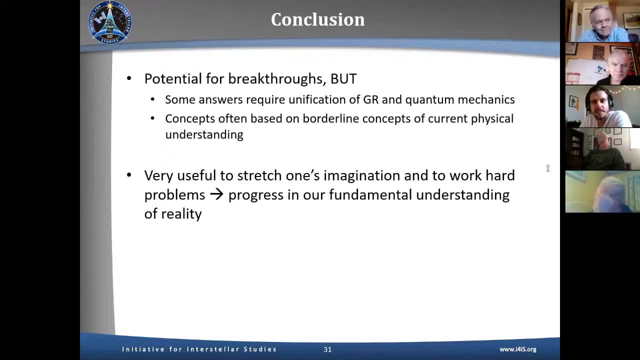 but uh, you know, you know we worry about the singularity at the heart of a black hole, while every single electron is a singularity unto its own. and you know the um, the idea that the um core of this paper of Wheeler back in the early 60s is that the bottom of an electron 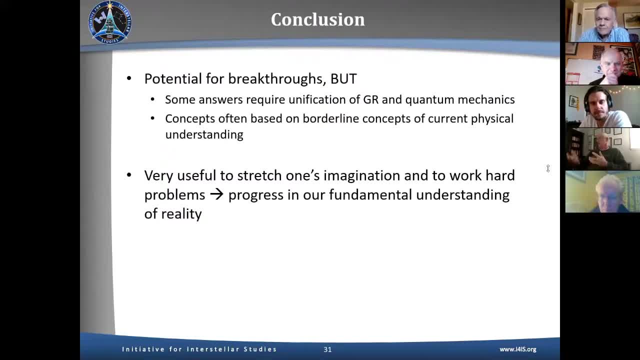 is actually the mouth of a wormhole and the um. you know matter and anti-matter is either you know the field lines going into a wormhole mouth or exiting, and that kind of ties in with some of the stuff that's been going on lately with the um. I want to get the words right. the um. 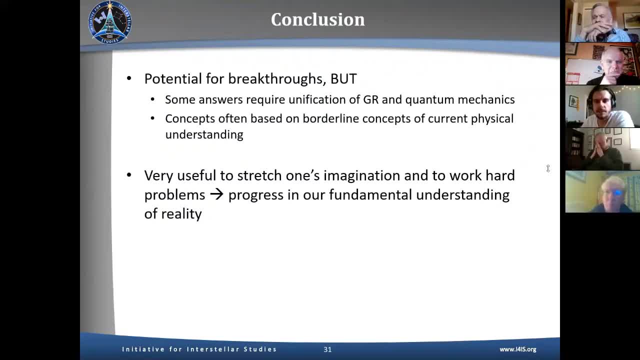 the, the, the quantum correlation in the um, you know the delayed choice type of experiments in that where um for what they're doing in the core of quantum computing. Dan and John, can I jump in there? just jump in there, because I think some of these very interesting um things at the edge of known physics are really interesting and we probably 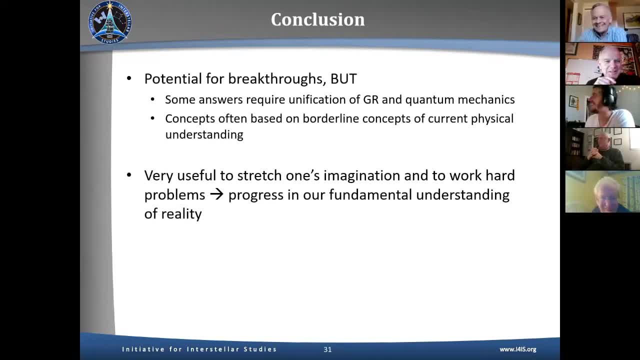 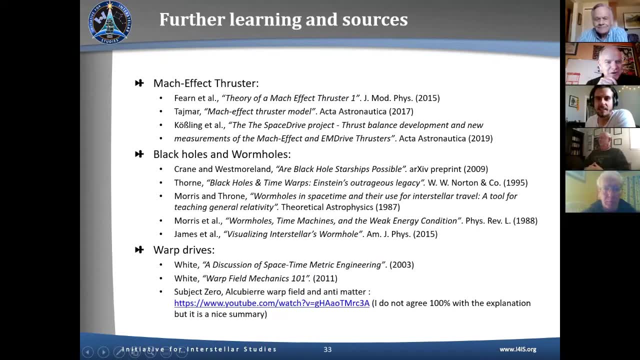 should be down the pub, uh, discussing some of them in more detail, and I'm very aware of the. you've only got a couple more minutes to go, so I wonder if David has got his hand up. David Fields, if he wants to ask his final question, the final question, then maybe you can get off to your lap to. 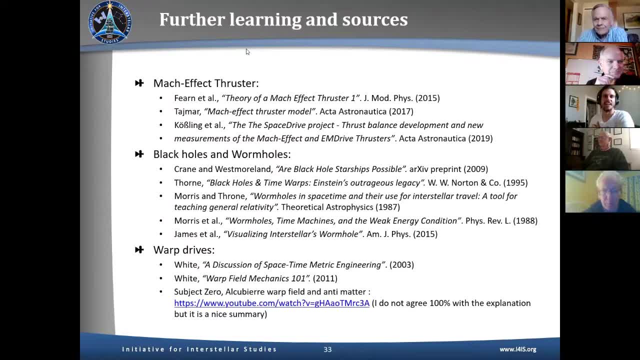 to sort out the waterworks. whatever it is, David, okay, yeah, thanks, Rob, the digital hand appears. that's like the thing in the bible. anyway, hey, Dan, nice presentation. thank you, uh, I got distracted because I got into what something John said and thinking about. the next thing we should explore is 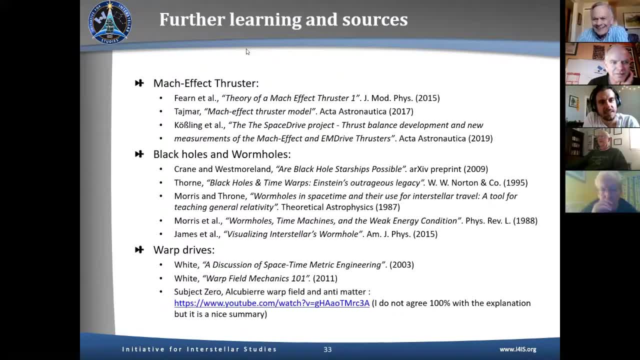 called the- uh, the inflation drive A little bit scary. my original question was: uh, you covered these types of drives here nicely, but you know they're, they're all going to be a little bit inefficient and whether that appears as as pulses of exotic particles or ripples and gravitational energy, or with a marker, just. 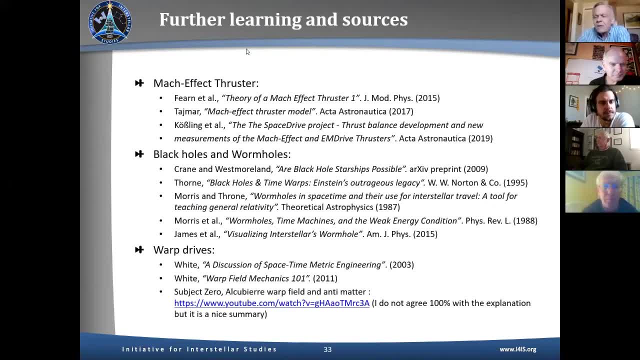 electromagnetic things. it seems like a nice opportunity to do steady research. so if, if you come across anything like that, you know that's got a characteristic frequency, um, or characteristic chirp or something like that might be a, that'd be a nice thing to think about. anyway, thank you, yeah. thank you, Rob. yeah, thank you, yeah, it's a. I actually never thought about. 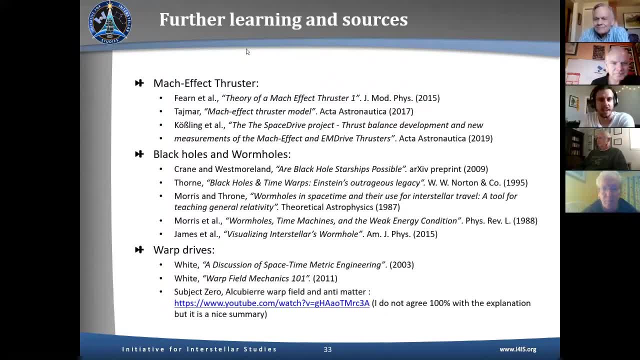 that that's a. that's a very good point. uh, yeah, I mean I mentioned this earlier- like the, the research in gravitate gravitational wave astronomy is, uh, I think, only in its infancy. uh, so it might be that we come across some very new things there, that. 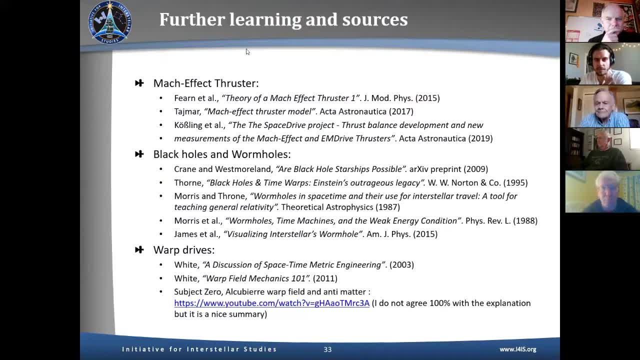 we have not expected and, of course, yeah, it's a very good point that we should always look out for other intelligences in the signal. um, you know, usually we can find a natural explanation, but, yeah, that's a that's an interesting prospect. um, okay, so there's one more question from uh, pat patrick. 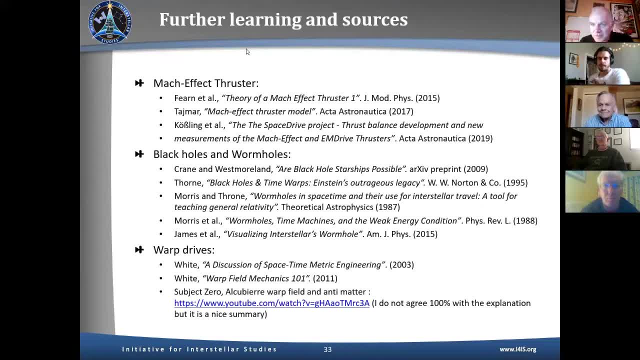 in the chat. well, I'm not sure. Sure, From my perspective, it does seem like we're getting slowly to a point where the unreconcilable differences in different fields are starting to pile up a little bit. Then again, a lot of developments in fields are also so deep and specialized that it's very hard to even hear about them if you're not really in the field. 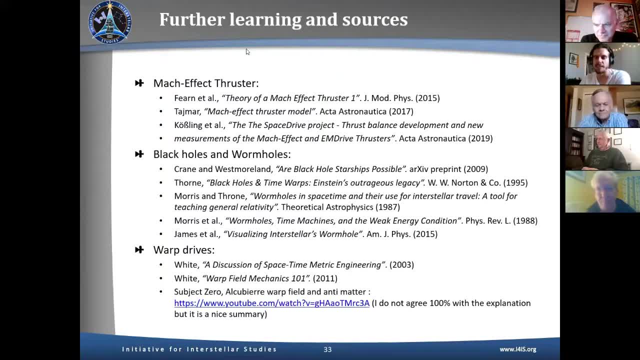 I personally don't like saying that we need another Einstein, because, yes, Einstein definitely was a great mind, but he also- I mean, the reason he was able to do what he did- was because there was so much work done before him And he was able, he was in the right position to take all of that and put his own mind to build something out of it. 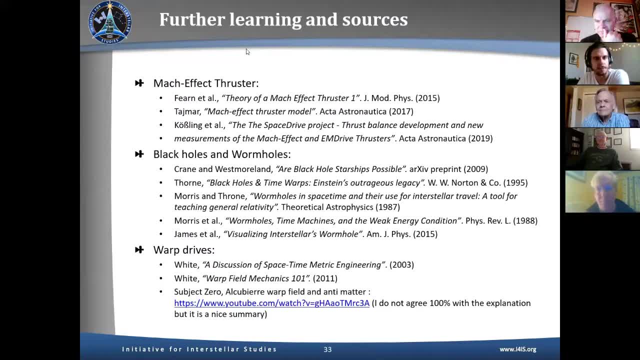 And I think that's how we should keep looking at it, Meaning that everybody should make as much contribution as possible And then, hopefully, somebody will eventually be in the right position to put it all together for the next step, John. so, okay, I might have to sign off after this, but before you say your thing, I just want to say thank you all for attending and listening, and I hope you enjoyed it. 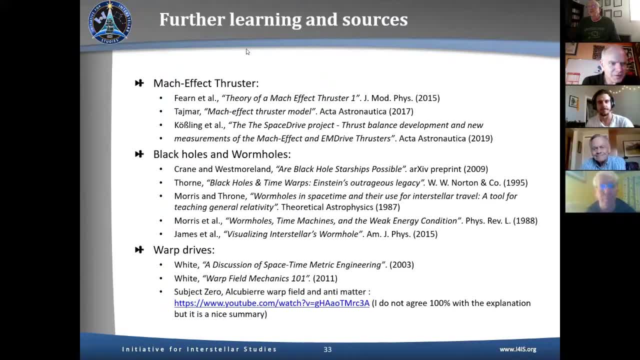 And yeah, go ahead, John. Yeah, no, just with regards to the Einstein. Actually, what I'd like to say is that I think it's a very important thing to do. I think it's a very important thing to do. 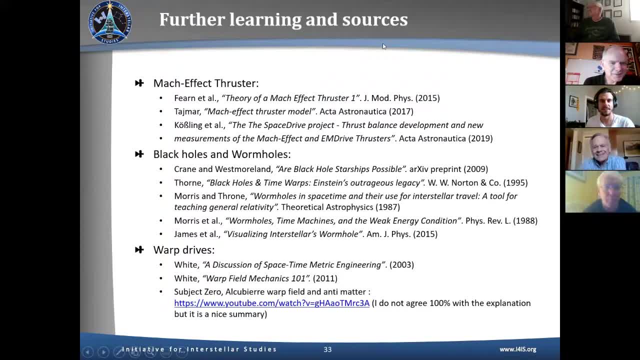 I think what I'd like to see is another pair of Wright brothers. Okay, They didn't have to invent new physics, They just figured out what was already there. Yeah, Yeah, true, Okay, I'll draw a close to the questions just now. 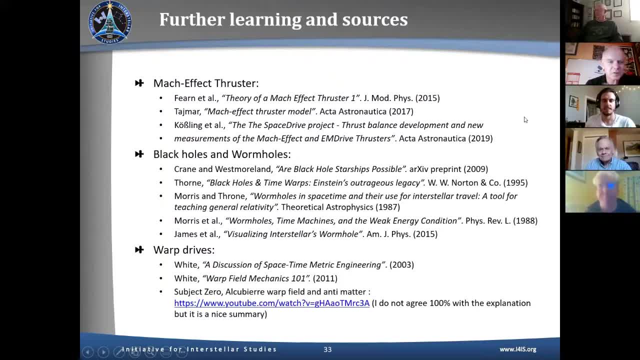 I know Dan has got the shoot off And I say thank you again, Dan, for that Very interesting It's all going to be. it's all been recorded And it'll. if, like me, I might need to watch it again. 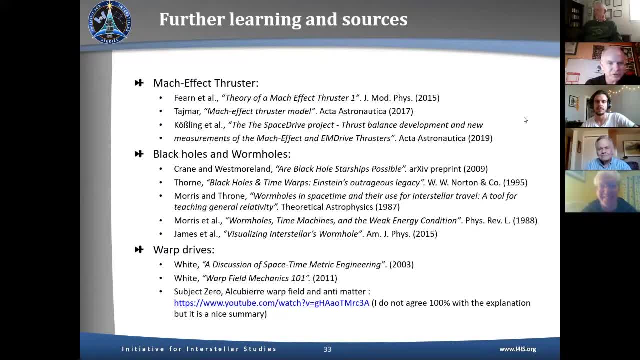 I'll watch it again through the website. It'll be on there in a week or so's time when the guys can put the video together. But thanks again for that, Dan. I'm sure everyone will. I'll say thank you as well.